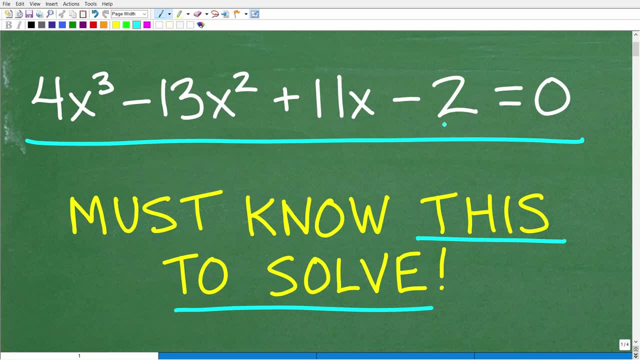 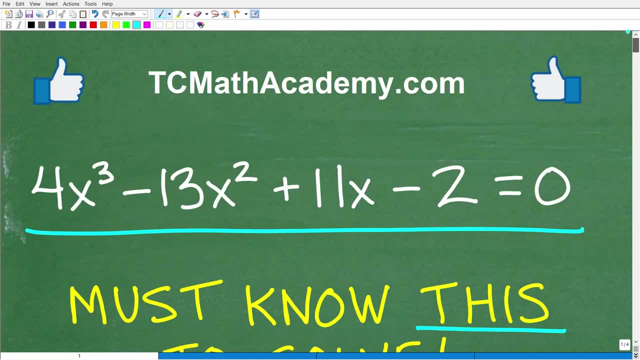 4x cubed minus 13x, squared plus 11x minus 2, is equal to 0.. That is the problem. Feel free to use a calculator, But if you can figure this out and solve for x, well, that would be super impressive. 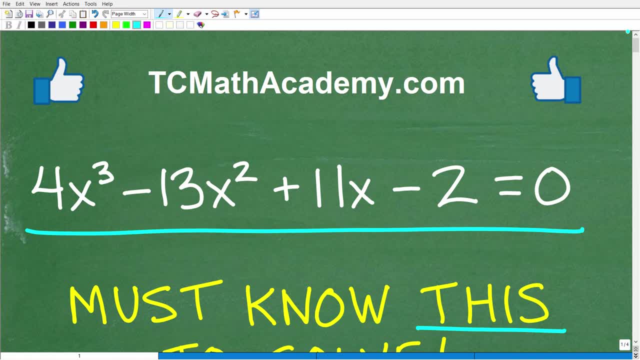 Matter of fact, if you have the answer, put that into the comment section. I'll show you the correct answer in just one second And, of course, we'll walk through all the work and steps that are necessary in order to solve a problem like this in algebra. But before we get started, let me 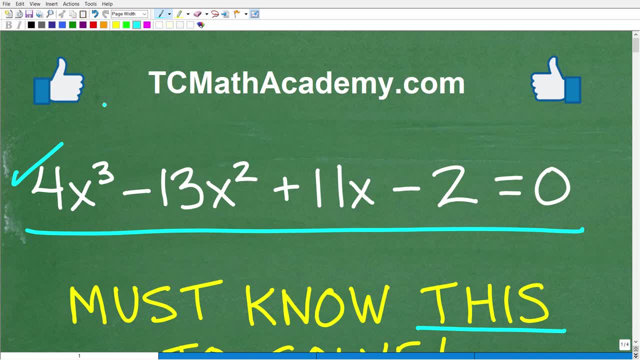 quickly introduce myself. My name is John and I have been teaching middle and high school math for decades, And if you need help learning math, well, check out my math help program at tcmathacademycom. You can find a link to that. 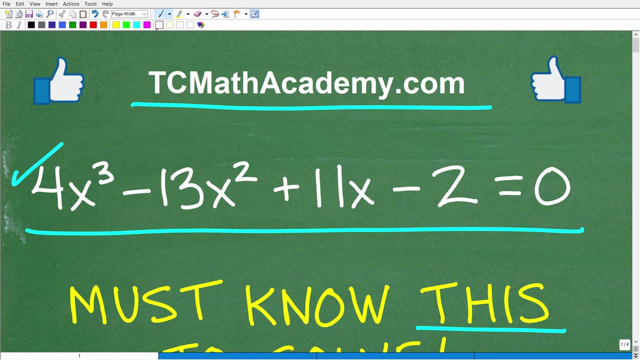 in the description below, And if this video helps you out, or if you just enjoy this content, make sure to like and subscribe, as that definitely helps me out. All right, now I'm going to be covering a lot of material in this video. I'm just going to basically be kind of summarizing. 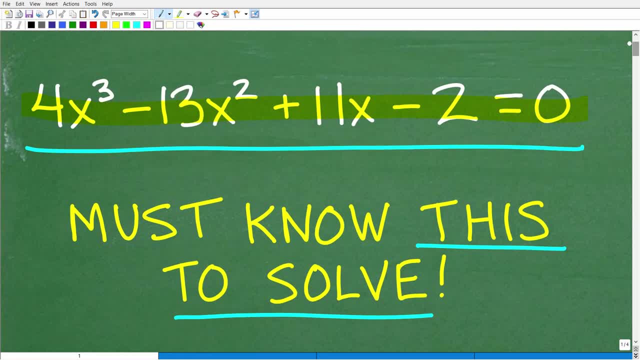 a lot of different concepts that you absolutely need to understand in order to be able to handle solving higher order polynomial equations. So, for example, if you were taking maybe a first year algebra course, you should be able to solve an equation just up to here. So, matter of fact, we'll just take this x cubed out for a second. 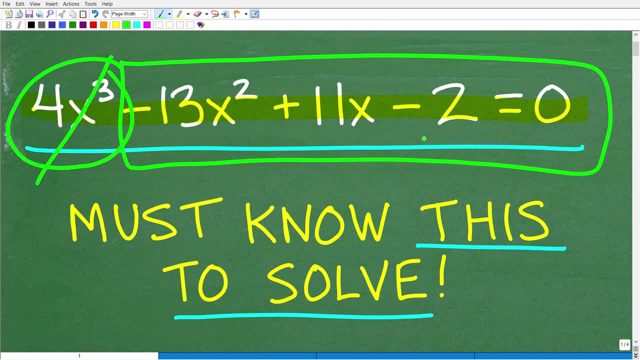 So this right here is a quadratic equation. So how to solve quadratic equations is a big part of what you learn in algebra, one first year algebra. But as soon as we kind of throw in another term here with a cube, all right, an x cubed situation, well, this is a whole different. 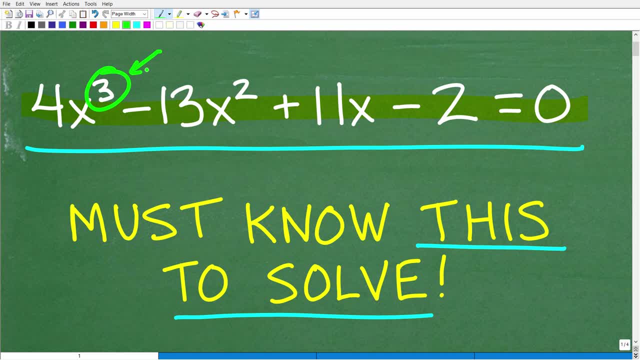 ballgame- Okay, really kind of ups. what you need to know- And of course, you need to know this As a matter of fact, you need to know much more than what this one specific thing is. So you may not have seen this. 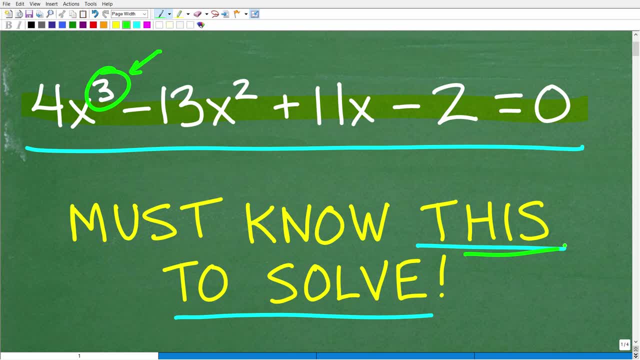 level of math. yet This is typically stuff that you will learn in algebra two, college algebra or pre calculus. So if you haven't seen this well, this is what you have to look forward to. Okay, so let's go ahead and take a look at the answer. So the answer to this equation is the. 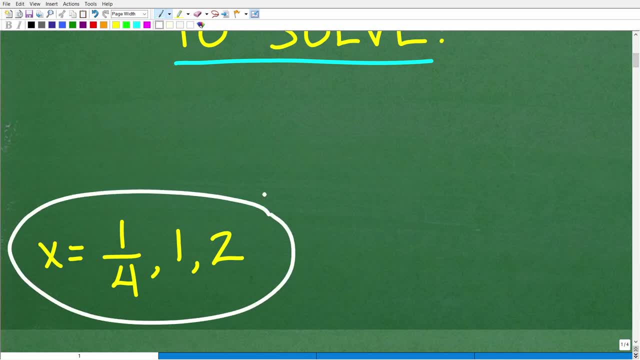 following: x is equal to one, fourth, one and two. All right now, if you're going to be able to solve this equation, you're going to have to take a look at the answer. So if you got this right, that is super impressive. Matter of fact, I have to give you a. 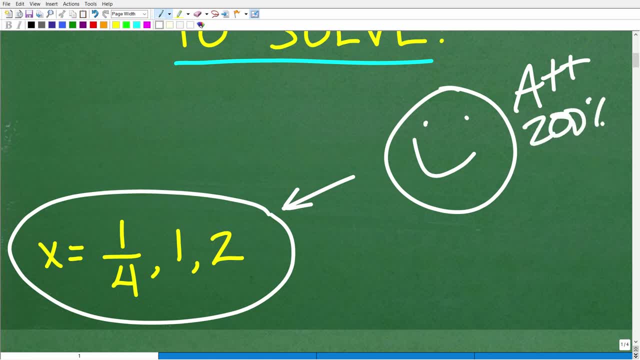 happy face and a plus plus a 200%. Matter of fact. I would just say if you were in my algebra two class I would say: just take the rest of the year off. I don't know how you got so smart in algebra. 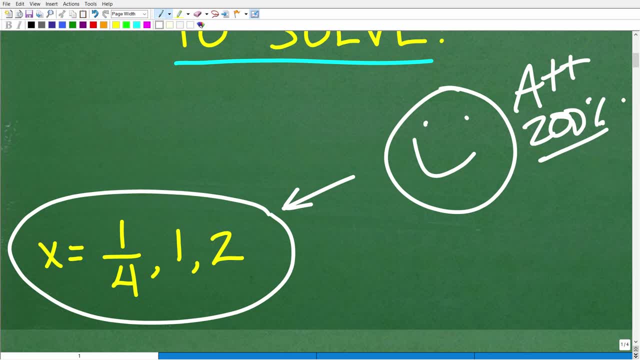 Maybe you're watching that guy on YouTube, But anyways, this is very, very good work if you're able to figure this thing out. Now, one quick thing about a calculator. A calculator could help you out. Matter of fact, using calculators at this level of math, you're going to be able to. 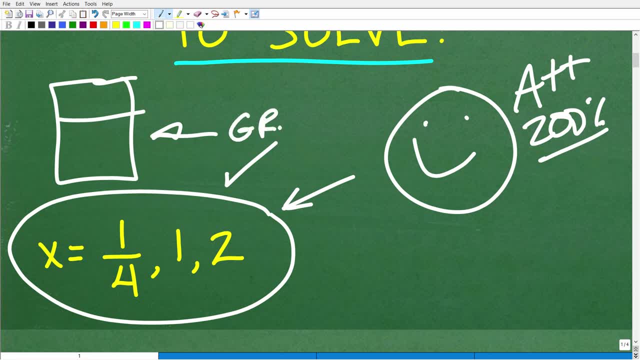 math is really important And if you have not invested in a graphing calculator, you know. if you really want to learn matter of fact, I can really spell graphing correct here- graphing calculator- you really definitely need to think about investing in one. So I'm talking. 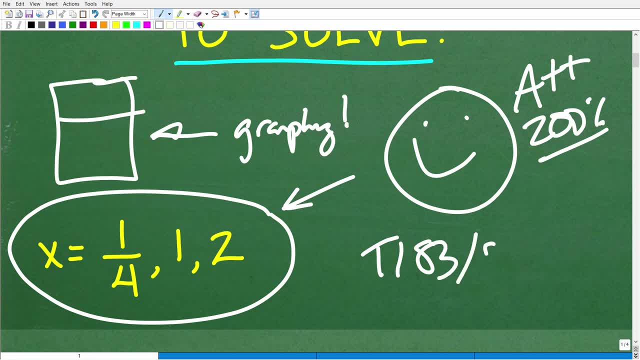 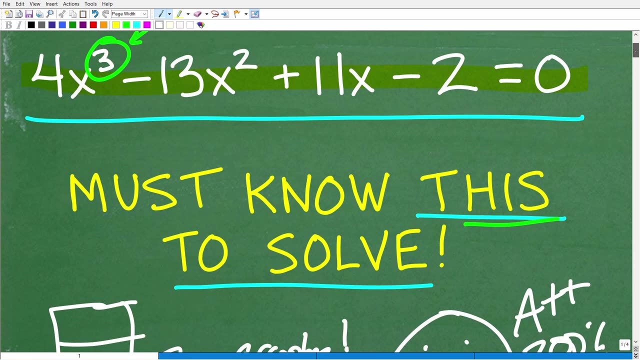 about calculators like TI-83, TI-84.. There's other types of graphing calculators. Usually they're going to cost you at least a hundred dollars, or maybe a little bit more. So these calculators are super powerful And one of the things that you can do here is to graph. 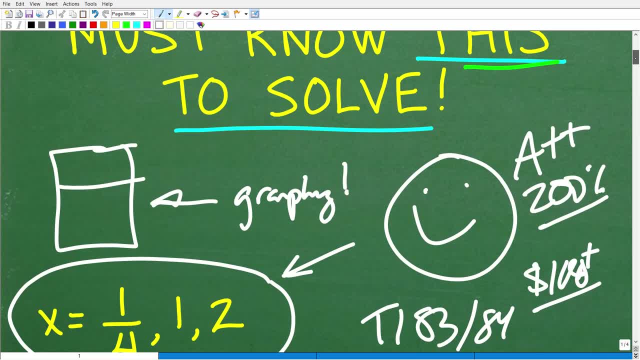 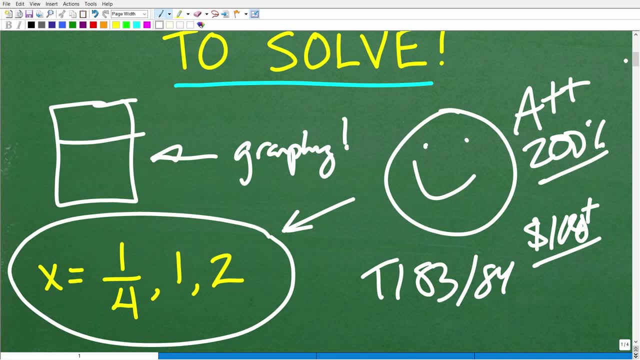 this polynomial function And the graph will give you a lot of clues on how to find the solutions. But you're not going to always be able to use your graphing calculator. You need to know the specific algebraic techniques, And that's what we're going to be talking about, And I'm going 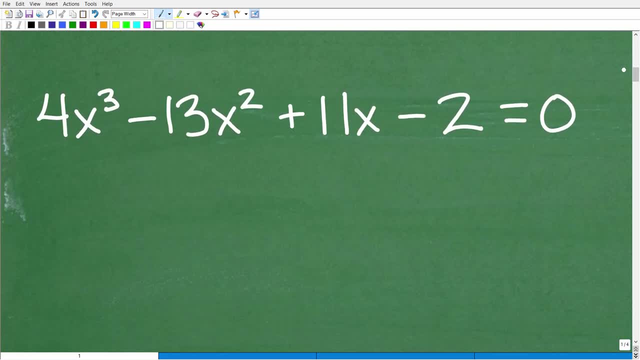 to quickly go through this, And this is not going to be all that quick of a video because we have a lot to cover. So if you don't understand anything, you know what I'm getting into because I am going to be going kind of quick. 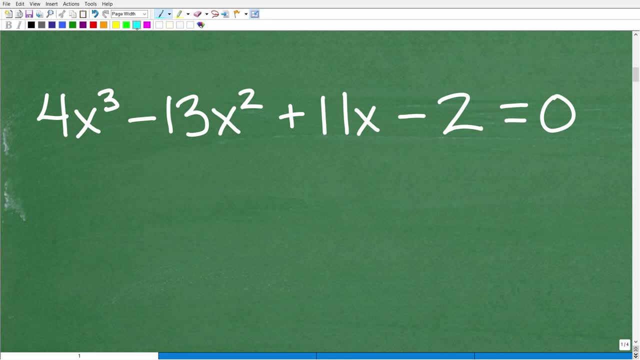 We're talking about multiple different sections and chapters of algebra concepts that you should master here. So if you need help with any of this stuff, check out my algebra two and or pre-calculus courses. You can find links to those in the description of this video if you need help. 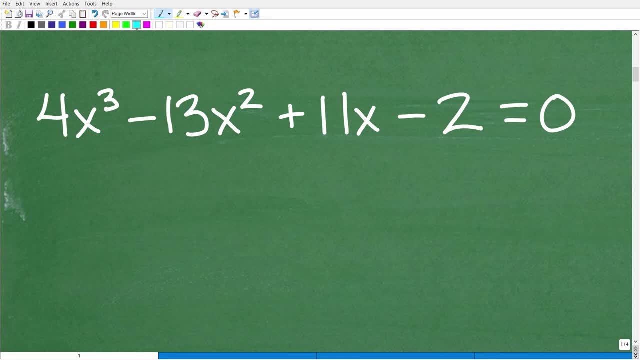 beyond this video, All right. So first things first. let's take a look at this equation from a kind of big picture standpoint, All right. So we're dealing with a polynomial equation. This is a polynomial, And why it's a polynomial. again, this is something you should know. 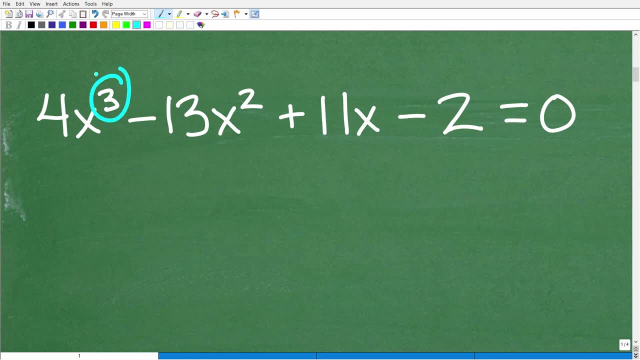 But it is a polynomial And it is a third degree polynomial equation. So we want to kind of consider this thing right here, which is the fundamental theorem of algebra And more or less the fundamental theorem of algebra. It's a pretty fancy theorem But it's an extremely important. 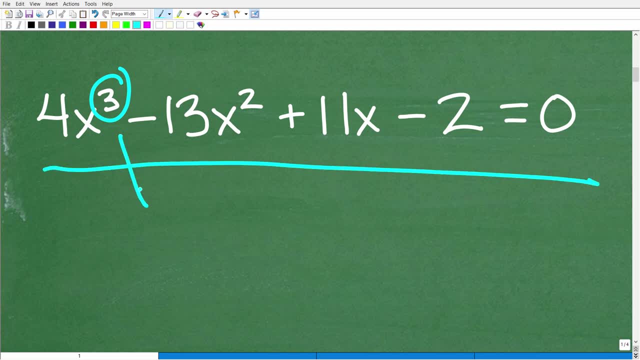 theorem And it says: hey, if you have a polynomial equation, the highest degree or the degree of that polynomial OK is how many solutions you're going to have. So this polynomial is going to have three solutions. Now, what type of solutions? Well, 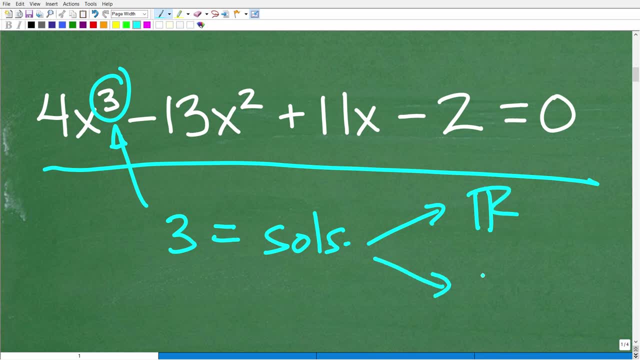 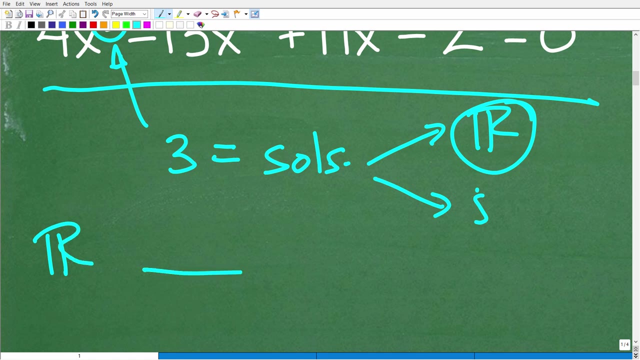 it can have real number solutions And it can have imaginary or complex number solutions, We just don't know. OK, But it will have three solutions. Now let's talk about real number solutions. OK, Now, again, these are things that hopefully you know. So the set of real numbers is: 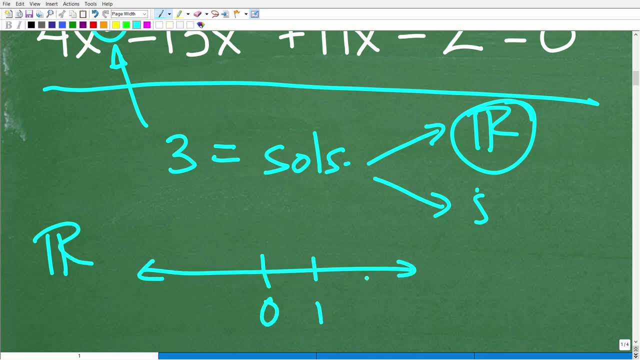 what Well it's all these numbers on the number line. So it's like 0, 1, 2, negative 1, negative 2.. So these are of course the integers, And then in between the integers we have fractions. We 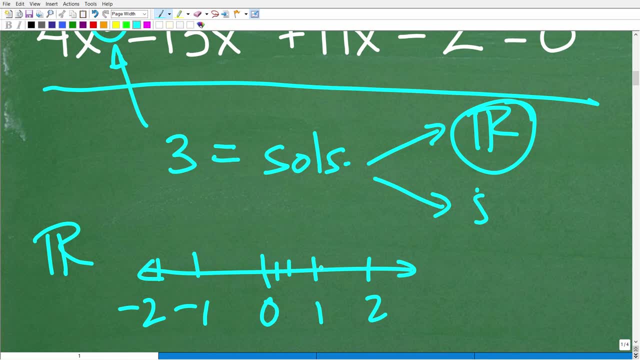 have rational numbers, irrational numbers, et cetera, et cetera. OK, So again, this is what real numbers are, And I want you to remember rational numbers. Rational numbers, Remember what rational numbers are. These are numbers that you can express as a fraction, So, for example, 2,. 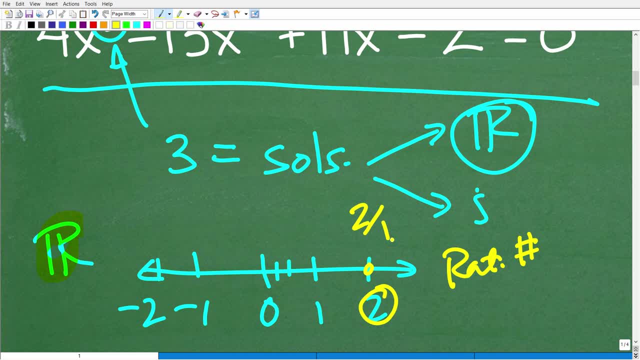 you can express as a fraction. Matter of fact, let me go ahead and just fix that definition. Rational numbers are numbers that you can express as a fraction of using integers. OK, So, for example, 1 half is a number that we can express as a fraction using integers. 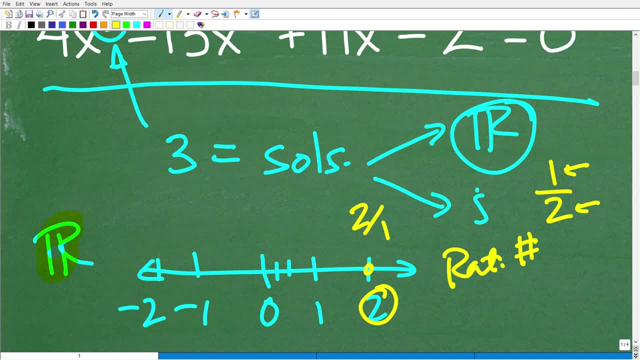 because a numerator and denominator is an integer. Negative 1 half is again a rational number, 7 is a rational number, et cetera, et cetera. OK, All right. So keep that in mind, All right So. 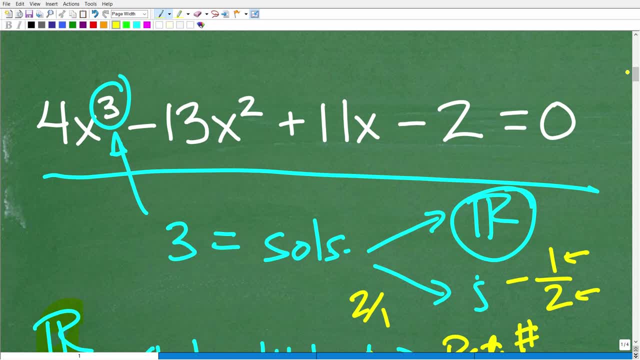 this is kind of the big picture in terms of facing an equation like this. We're like: all right, we have a third degree polynomial equation. There's absolutely going to be three solutions. I have no idea if they're going to be a real number and or imaginary or some sort of combination. So we need 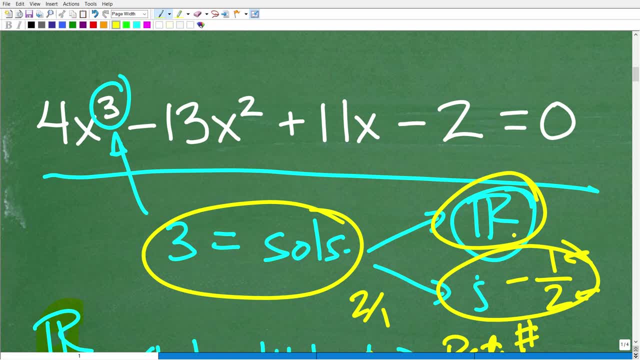 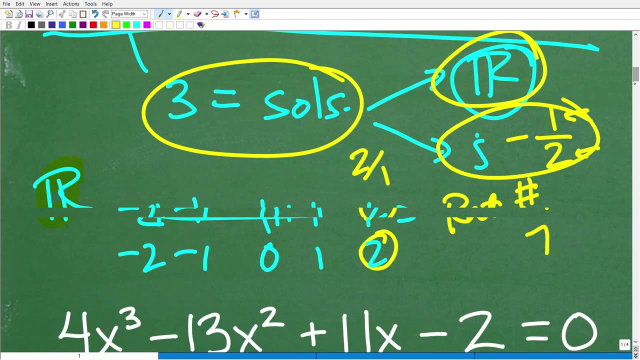 a way to kind of get started here. Now again, if you had a graphing calculator, that would provide a tremendous clue on where some solutions could be. Now you could even graph this by hand, but that's a lot of work, So we need some other tools, And that's what we're going to get into. 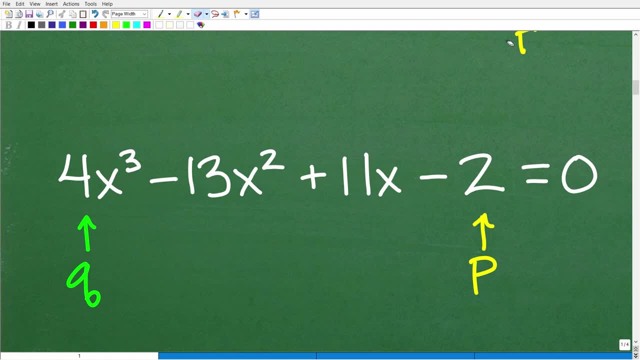 here, OK, So I'm going to show you something that you absolutely need to understand at this level of math. And before I show you this, we want to make sure that our polynomial is written in standard form: highest to lowest power, and it's set equal to zero. OK, So of course, we already 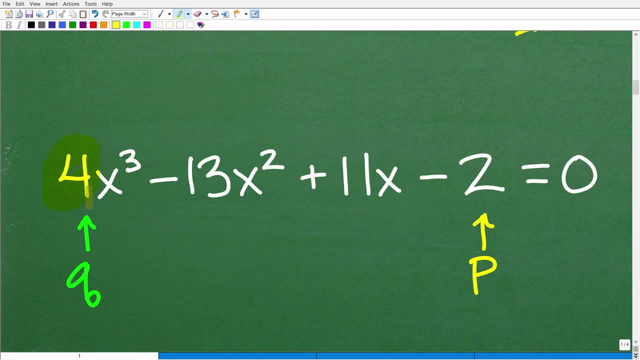 have that situation Now I want you to pay attention to the leading coefficient. OK, So the number in front of the leading term is 4.. That's going to be our Q And you're going to be like: what is Q? 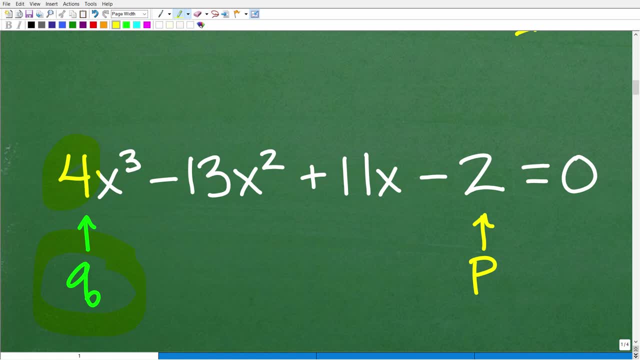 Stand for it. Well, I'm going to show you in a second, but just know that this is going to be our Q, And then this little negative 2, our number is going to be our P. OK, So we're going to be using. 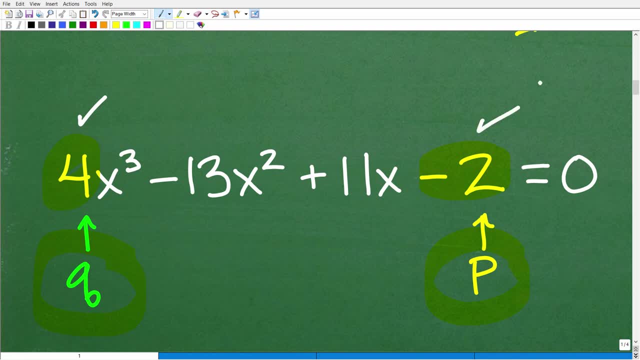 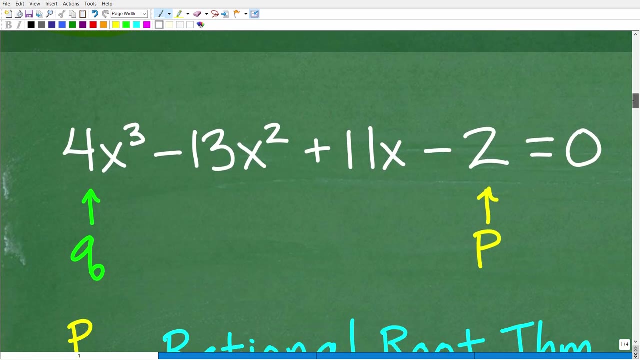 these two things to give us a clue on this: possible solutions for this equation. All right, So again, we have to be in standard form, And our leading coefficient is Q, And our last number here is going to be P. OK, So what am I doing here? Well, I'm talking about an extremely 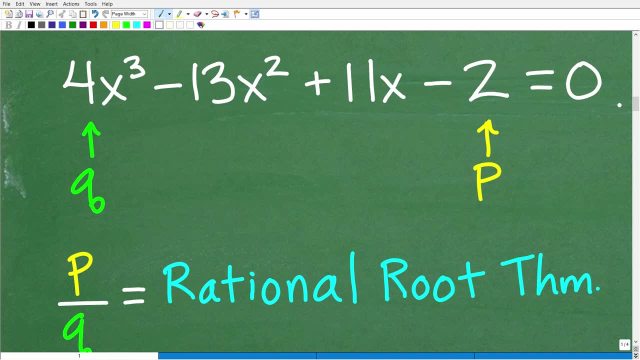 important thing, And this is what I was alluding to in the title of this video- You need to understand this one thing in order to solve this equation, And this is called the rational root theorem. Now there are even other theorems. This is a big, huge topic in advanced math. 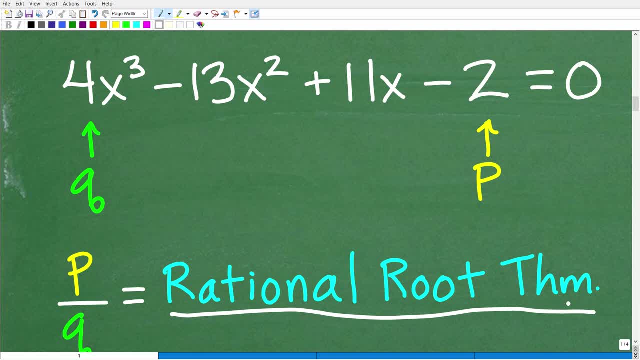 how to solve polynomial equations. There's other theorems I could kind of get into that will give you more kind of additional clues on where the possible solutions and roots lie, But this one is the rational root theorem. OK, So let's just take a look at the name before I even tell you. 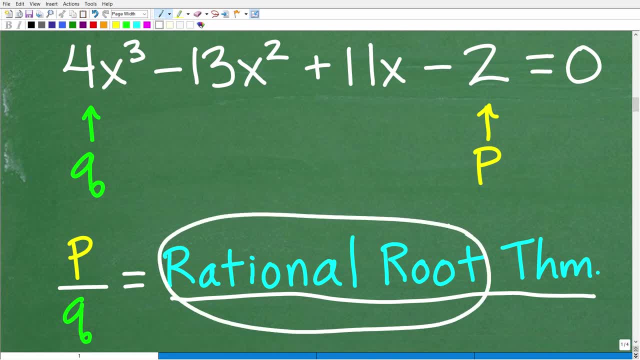 how to you know how it works? What is this name right here? Rational root. Well, we're talking about rational solutions. So a root is an answer, It's a solution to our polynomial equation. So we could even kind of name this rational solutions theorem. So what is rational again? Well, we're 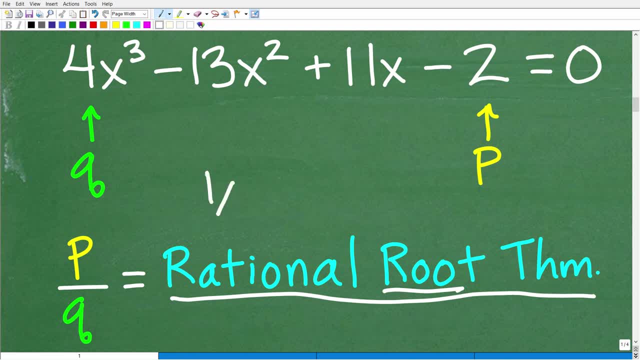 talking about rational, real numbers. We're talking about numbers that can be expressed as a fraction. So we're talking about numbers that can be expressed as a fraction. So we're talking of integers, things like one, half or one, fifth or two sevenths or eight, nine, one, et cetera. 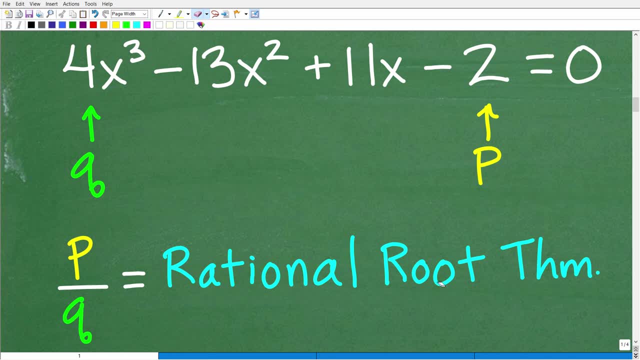 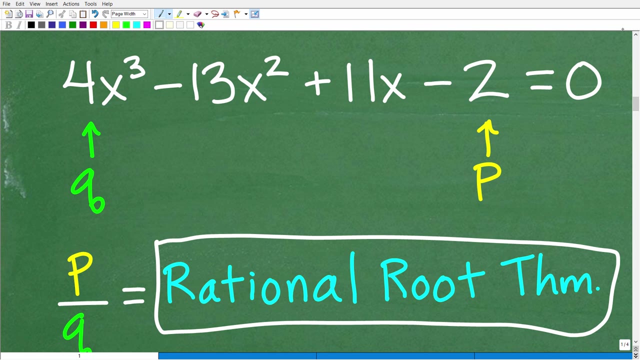 et cetera. OK, so the rational root theorem is basically the following: OK, now we're going to look at how to actually use the theorem, but let's just kind of understand its application or what it represents. So, as I indicated, this polynomial- OK, this polynomial equation- definitely has three. 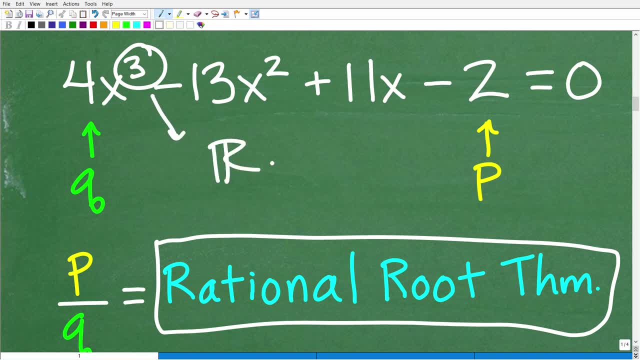 solutions. Now, you could have some real number solutions. Now, if you do have some real number solutions, you can have irrational numbers- OK, things like the square root of three, things like that. Or you could have rational numbers, which is actually. 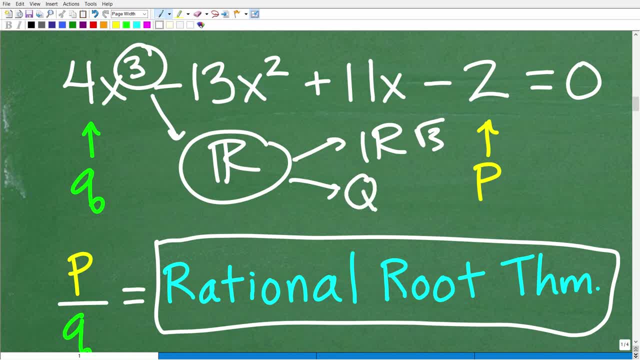 represented by this big old Q. OK, so Q, which is the set of rational numbers. Now, if this polynomial equation does have rational numbers as solutions, it's going to be part of a list that we can create. OK, so, in other words, we can determine. 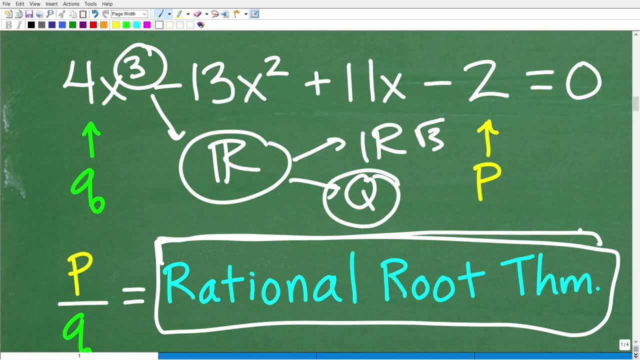 and find any possible rational roots that this polynomial may have in advance. OK, and this is going to have tremendous advantage for us in order to solve this polynomial equation Right. So again, we don't know if this polynomial equation has any rational roots, but if it does, it's going to be. 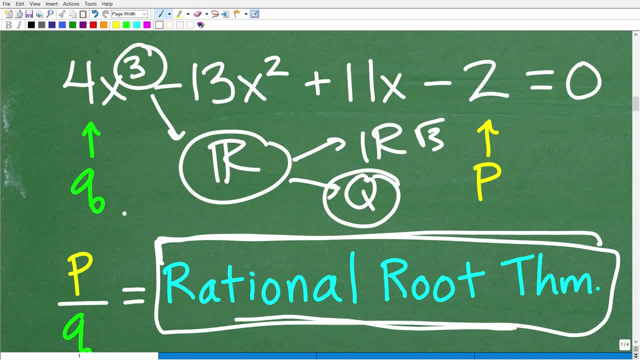 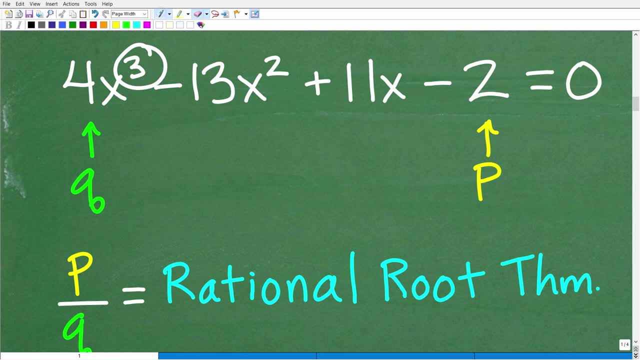 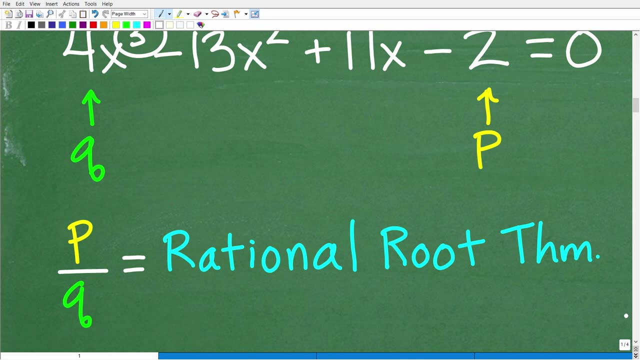 part of a list that we can build using this P and Q stuff. All right, So you know. you have to understand the whole purpose Of the rational root theorem before we actually start building it. So again, one more time, just to be extra redundant: We don't know if this polynomial equation does have rational roots. 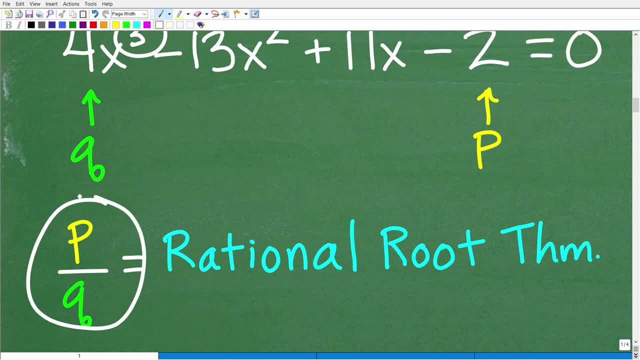 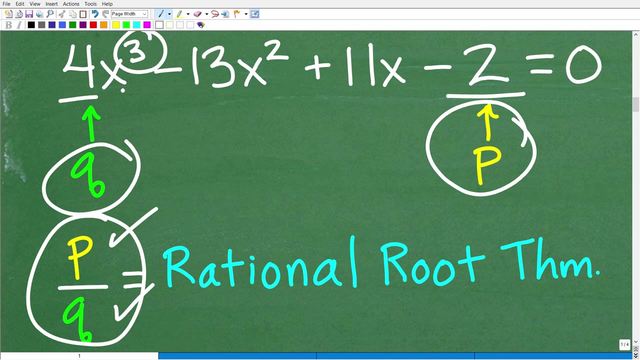 but if it does, it's going to be part of this list of possible solutions and we can build using this. P and Q, All right. So what is the P and Q business? Well, P is this number, this last number. in this particular example, it's negative two and Q is our four. All right, So the 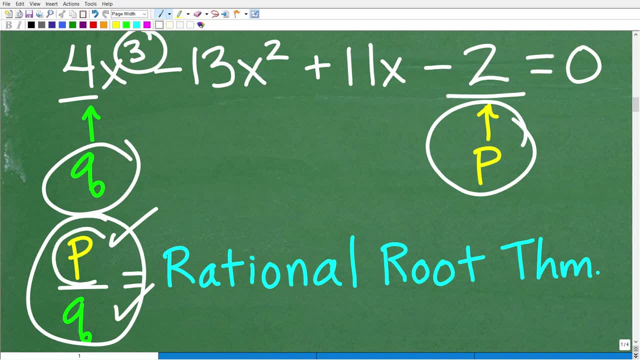 rational root theorem basically says this: We're going to take a look at all the factors of P and we're going to divide it by all the factors of Q and we're going to end up with one big list of possible rational roots. OK, so we really kind. 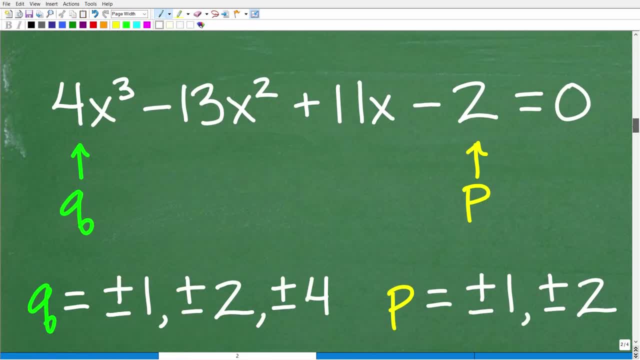 of have to see this in practice for this to make sense. So let's going to take a look at that right now. OK, so we have our P and Q. Now let's go and take a look at the factors of each of these. 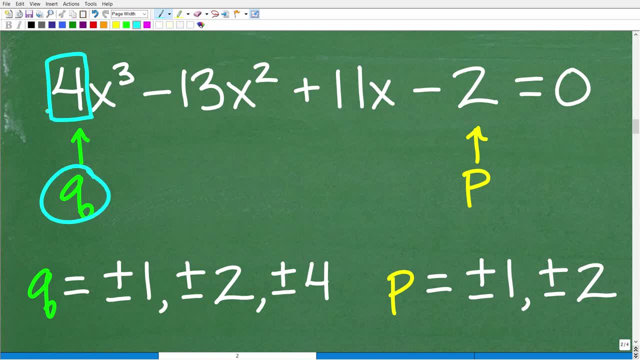 things right now. OK. so what are the factors of four? OK, well, it's one times four, right? Or we could have a positive one. I'll just list this out for this first example, because there's a lot of work here. So one times four, OK, is of course four, But so is a negative one times negative four. 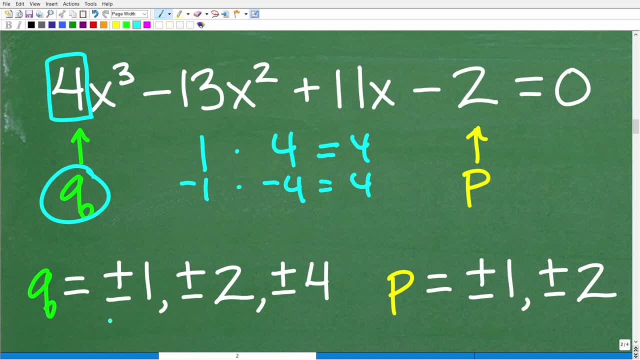 right, That is a positive four. So factors of four, OK, is positive negative one and positive negative four. But we also have two times two or negative, two times negative two. So any time you look at these factors with the rational root theorem it's always going to be positive and 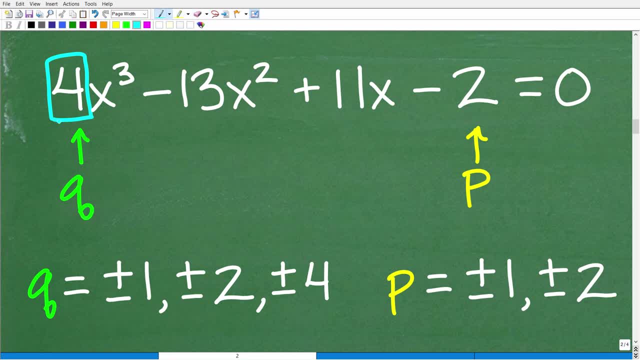 negative, right? So just think of the actual factors. Look at the number, like: OK, one and four and two times two, So it's always positive and negative. So the factors of this number, Q is positive, negative, one positive, negative, two, positive, negative, four. OK, so now let's go to. 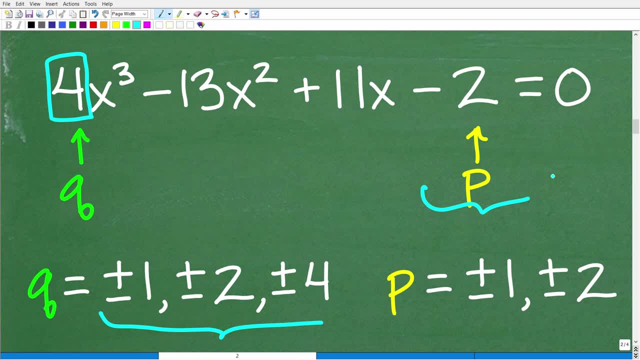 list out the factors of negative two. Again. you're just going to just get in the habit of listing the positive and negatives for each of these, So it's going to be one times two, or positive, negative one, Positive, negative, two. OK, so these are our factors of P and Q, And remember the rational. 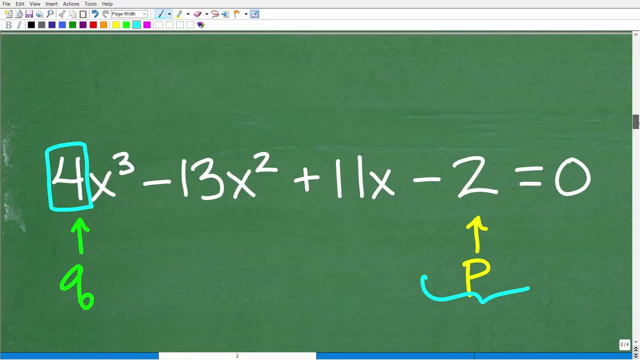 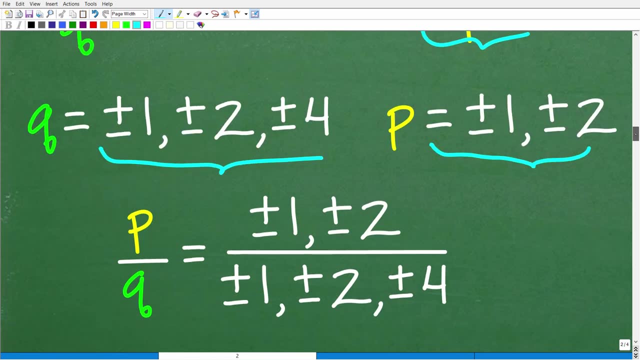 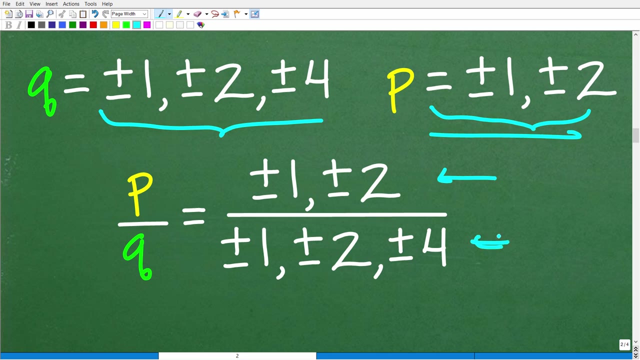 root theorem states that we need to divide these, So this can be a little bit confusing if you've never seen this before. Got to be very careful here. So now let's divide these two factors. OK, so P divided by Q: We're going to divide all the factors of P by all the factors of Q. 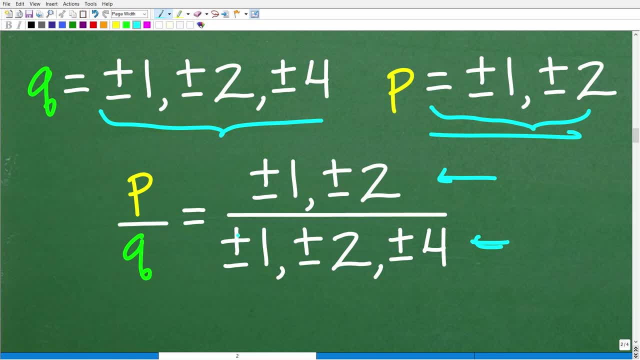 All right, so positive, negative, one, And then you're going to put a comma just like this: positive, negative, two, Divided by positive, negative one. positive, negative two, positive, negative, four. OK, so now we're going to have to look at each one of these and actually kind of figure out the actual solutions We're 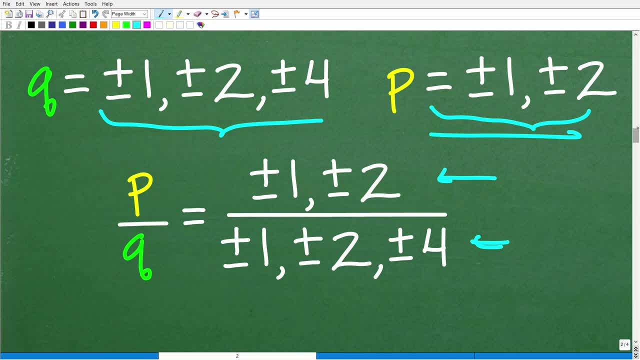 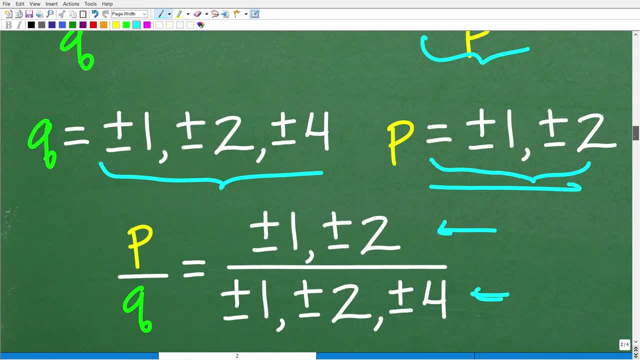 going to have to start doing some division here, And you're probably saying, hey, Mr YouTube, Math Man, this is a lot of work. Yes, it is a lot of work. As a matter of fact, this is actually a pretty easy problem to do when it comes to the rational root theorem. So let's go ahead and 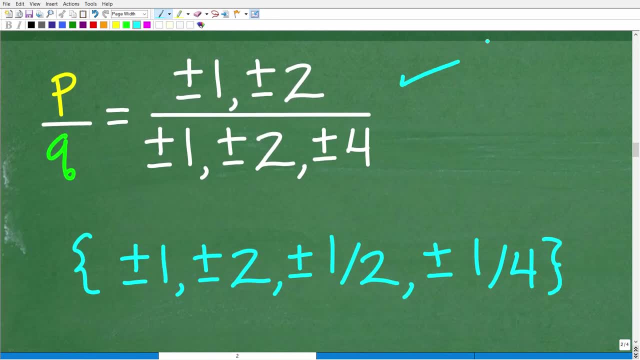 build our final list, All right. so first things, we have to get all our factors of P, all our factors of Q, And now we have to start kind of building out all the possibilities here. So let's start with one, OK, so we're going to take this one and we're going to divide it into this and 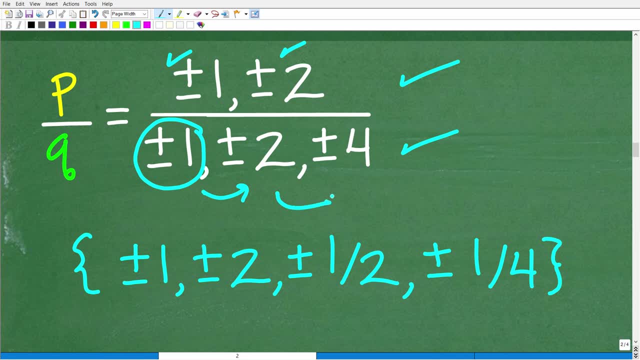 this. OK, then once we're done with that, we'll move on to two, and then we'll move on to four. Right, because we're doing division here. So what are all the possibilities? when we divide by positive, negative, one, So just go, one divided by one. Well, that's going to be a positive, negative. 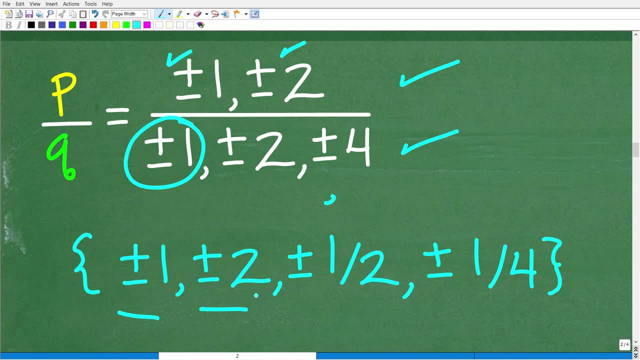 one. Two divided by one- Well, that's going to give me a two divided by one. So that's going to give me a two divided by one. Of course is two. OK, so we're done with one, All right, So now we're going to scoot over. 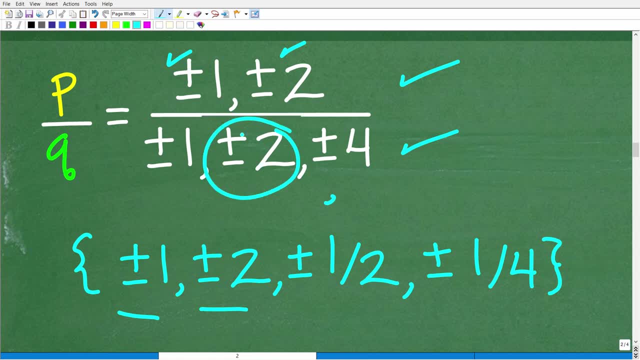 and take a look at two. OK, so two divided by one is what That's one half, Right? So our one divided by two- Excuse me, One divided by two is one half, And then two divided by two is one. We already have it in our list, OK, so we don't have to write that again. 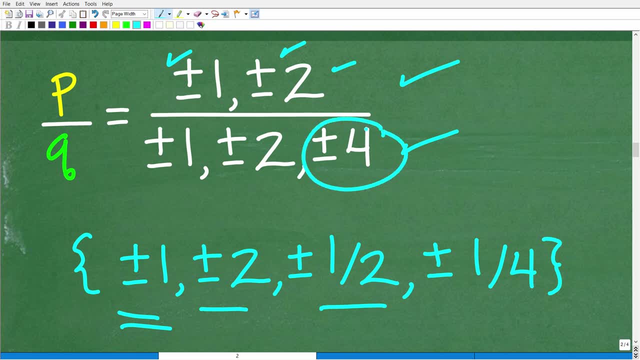 So now that we're done with that, let's move on to four. OK, so one divided by four is one fourth. Two divided by four is one half. OK, so one half we already have in our list, We don't have to write it. OK, so we've done every single combination of P. 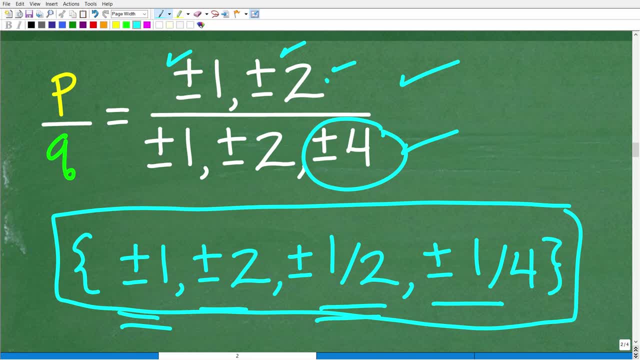 divided by Q. Again, P and Q are the factors of these numbers. And what are we looking at here? Well, if our polynomial equation has rational roots, they will be amongst these numbers right here. Now, it's very well possible that none of these numbers are solutions in our polynomial equation. 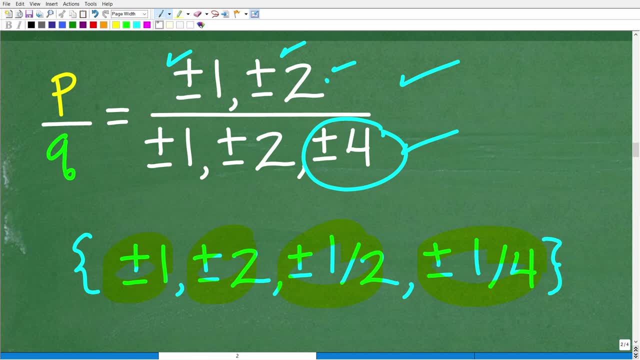 But if we do, if we're lucky enough to have a rational solution in this polynomial equation, it's going to be one of these numbers: It's going to be a positive, one, negative, one, positive, two negative, two, positive one half, negative one half and positive one. fourth, and 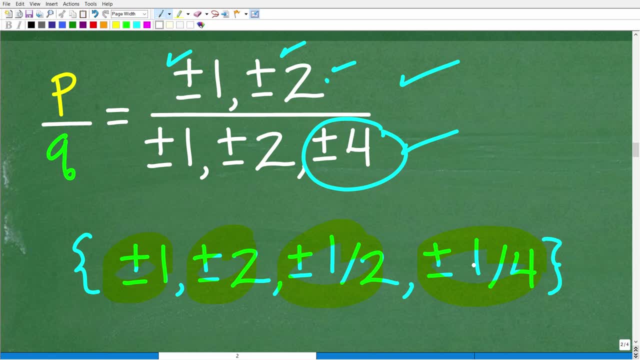 negative one. fourth: OK, so now that we have this possible list of rational numbers, what we want to do is we want to use these numbers to see if any of these are solutions, because if we can find solutions to at least even one, well this is going to really unlock how to solve the rest of this equation. 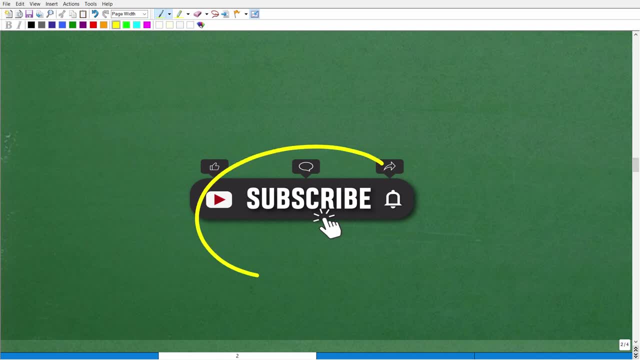 All right. So let's go and take the next step, which, of course, is having you quickly subscribe to my YouTube channel. You might be thinking to yourself: boy, Mr YouTube Math Man, it's a lot of work to put together a YouTube video like this. 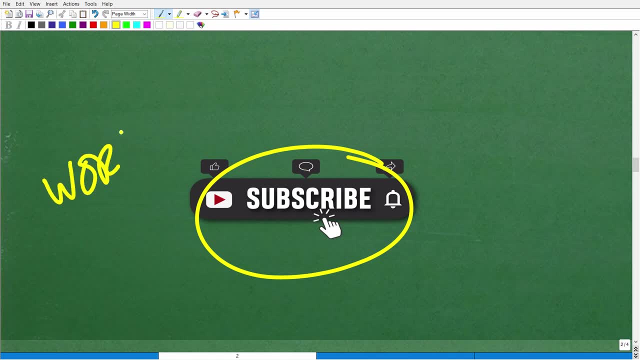 Well, to me it's not really work. OK, I love what I do, which, of course, is teaching math, But at this level of math, or anything like that, I'm going to be able to solve this equation. But at any level of math there's a lot of information And a lot of people get frustrated in math because they're like I'm bad. 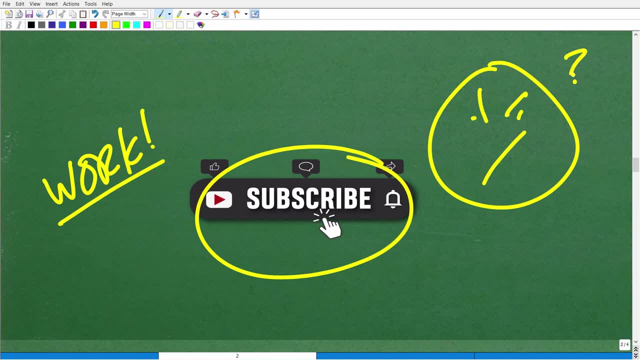 Well, you know what They? it's one or two things are happening. Either they haven't put in or they're bad at math, And that's what I meant to say. They haven't put in the work. You know, learning math, especially at this level of math and beyond, requires a lot of work. 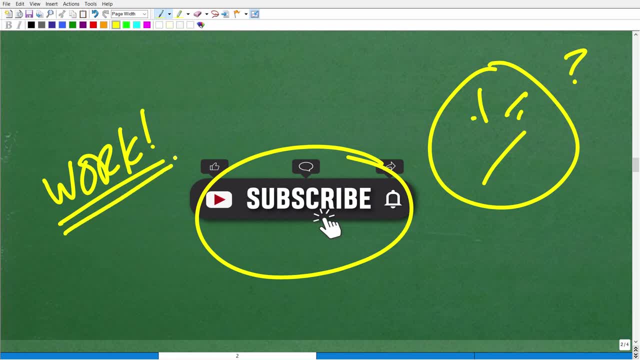 It requires effort, And you know you might think you might be thinking to yourself: well, I'm not smart enough. That's not the case at all. But you do have to ask yourself: are you working? Are you working hard enough? And if you are working hard enough, well then, the second piece of the puzzle that you need is great math instruction. 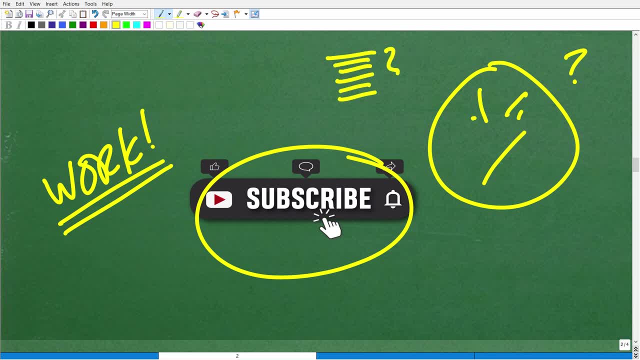 There's no way you can just do a quick review. A lot of people get deceived that they're learning math Like: OK, I quickly understand the rational route there. Well, there's a lot of little moving parts and details that if you don't understand, you know it's going to get confusing. 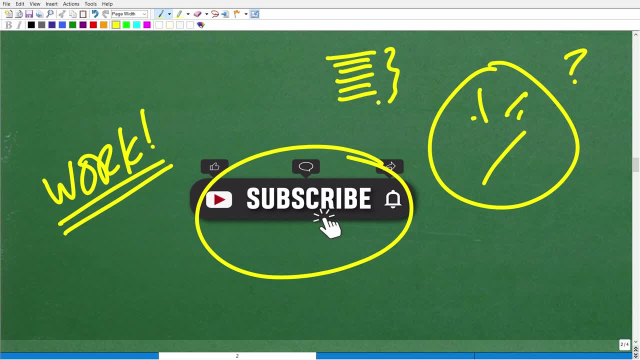 And the way I like to teach math is to break things down step by step by step. So if you're frustrated with math, well then, check out my full- I mean math- courses. you can find links to those in the description of this video and at this level of math. 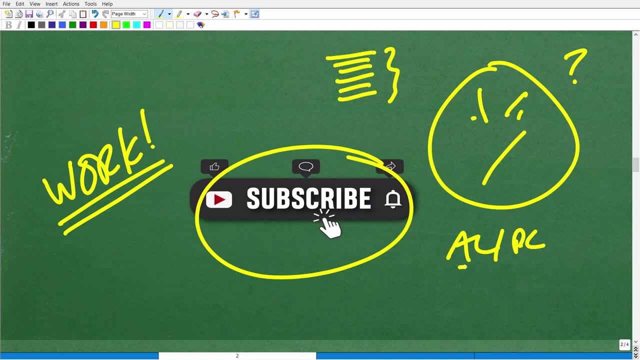 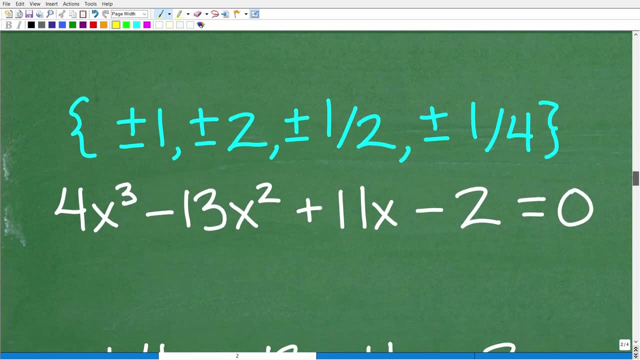 Again. you want to check out, like my Algebra two and or pre calculus course, All right, So let's get back to this problem because we have a lot more work to do And here is our list of possible rational solutions. Now the next part of this problem is a pretty fun part. 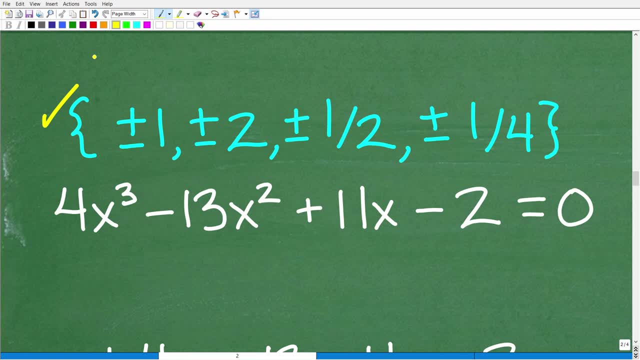 So what we're going to do is check these solutions to see if any of these are actual answers. Now, When we talk about the rational root theorem: Right, So a root. another word for this is zeros. That's pretty much all synonymous with solutions. 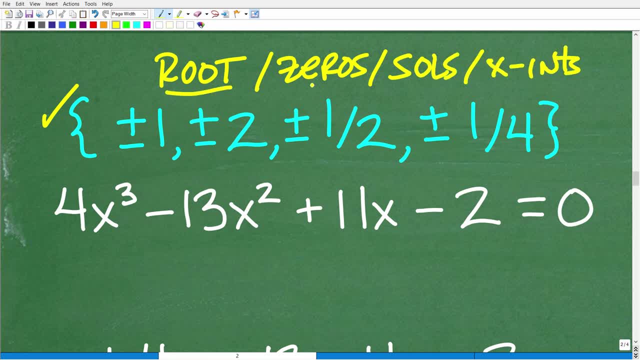 We can even throw in X intercepts as well, But a root of zero is, in fact, a solution to like a polynomial equation. OK, so how can we check these numbers to see if, in fact, they are solutions? Well, what you could do is take- let's take, for example, positive one- 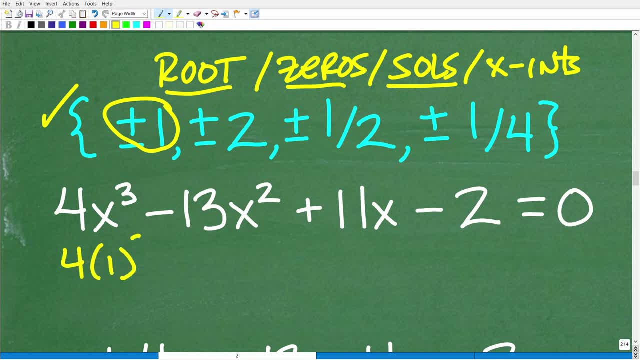 Let's check this. Well, you could plug in one for X, Right? So we would go like this and we just do all this number crunching right here to see if we did all of this. If, in fact, if it turns out to be zero and zero is equal to zero, then one is in fact a solution. 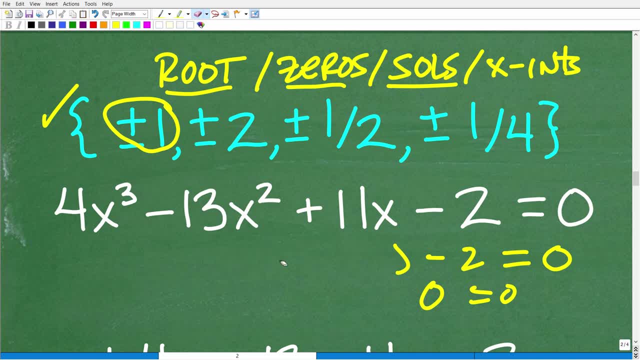 But this is not the way you're expected to kind of check these solutions. You could check them this way, but this is the long way. There is a much better way, And it brings me to another thing that you need to know at this level of math, and that's called. 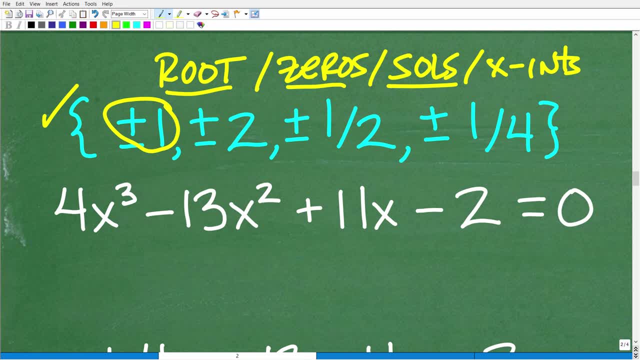 A polynomial division, specifically synthetic division, is a shortcut way to check to see if in fact, you have the correct roots. Now that's a other big deal. There's. there is the remainder theorem. This is a big, big topic in math. 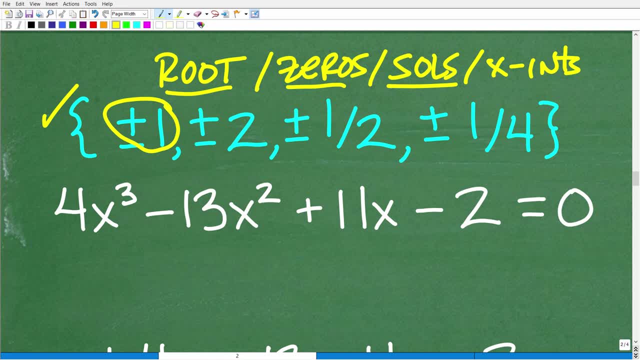 So, again, check out those courses that are referenced if you are confused about this. But let's go and take a look at how we can check these solutions using something called synthetic division. It's super cool, And what we're going to do is set up a thing that looks like this: 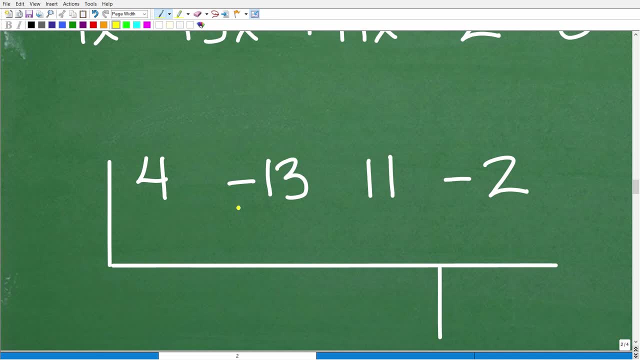 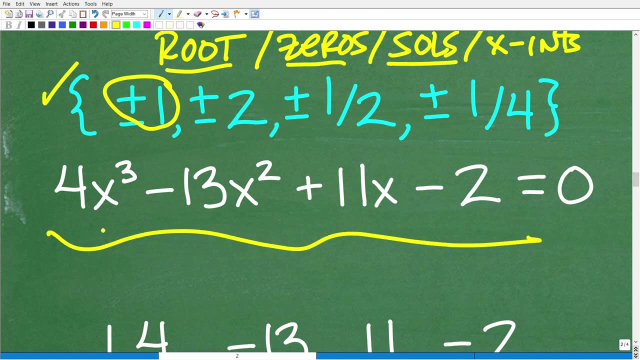 All right. So you got like an L Type of bracket. And then these numbers for negative thirteen, eleven, negative two are the coefficients of our polynomial. And notice, we have our cube or four right here first, And this is in standard form. 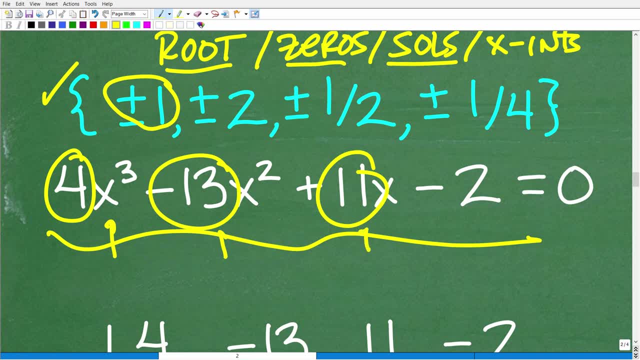 Negative thirteen, That's in front of our X. Eleven, That's in front of negative thirteen in front of our X. squared Eleven is in front of our X, And then negative two is the number. Now, if we were missing any terms here, you would have to put in a zero. 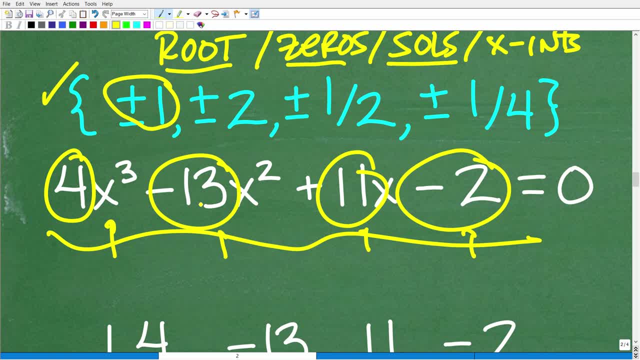 Again, I'm trying to explain something that really requires like a full Lesson, but I think most of you kind of get the main idea. So we're looking at all the coefficients of this polynomial in standard, standard form, So highest to lowest power. 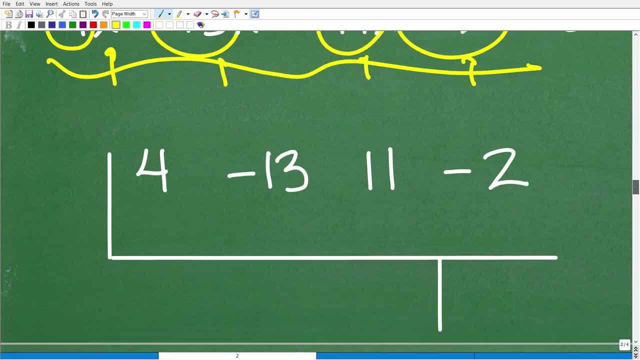 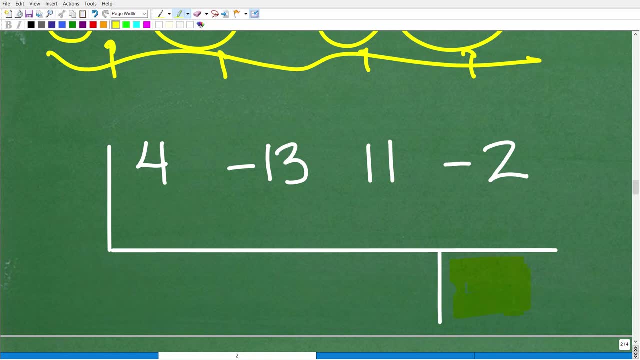 OK, so here we go. So we have four negative thirteen, eleven negative two, And then we're going to put a little line down here, because we're going to specifically be looking at this right here, which is going to be the remainder. 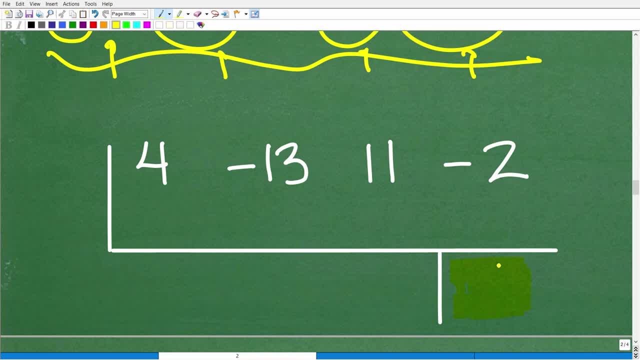 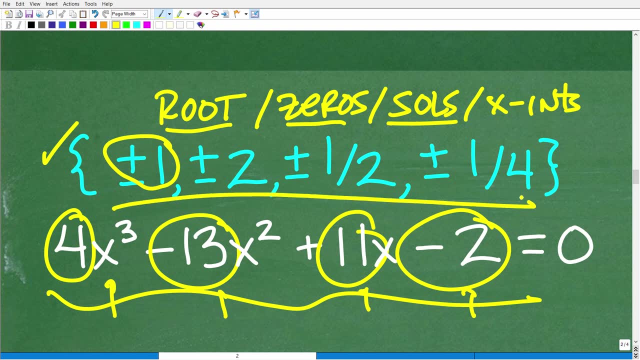 All right. So this is a awesome little technique. Again, we're going to be doing synthetic division, All right. Now what's the whole point Here? Well, we're going to check these numbers to see if any of these are in fact solutions to our polynomial equation. 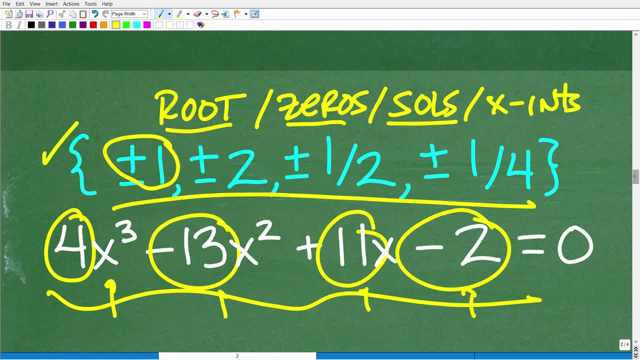 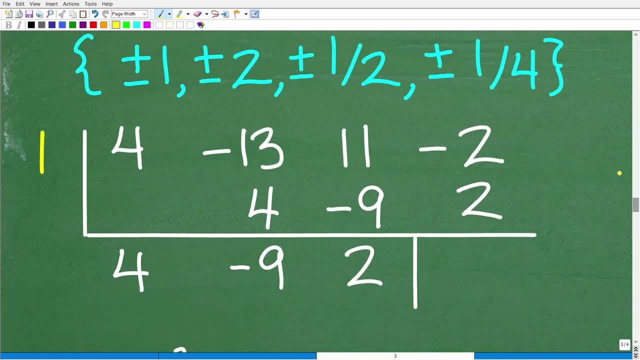 So we're just going to start with one and we'll work our way through the list. I'm not going to do all of these, but I am going to do a few so you can get the main idea, All right. So let's go ahead and start with positive one. 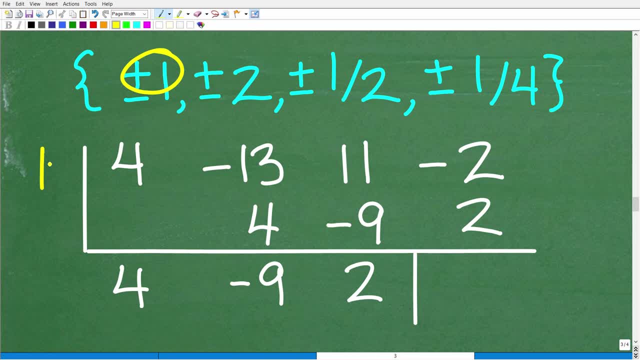 All right, So I'll start with positive one. So I'm going to put a one just like this, And this is how this technique works. OK, so your first number came. in this case, It's for you: Drop down Now. I already did the work here, but I'm going to explain it. 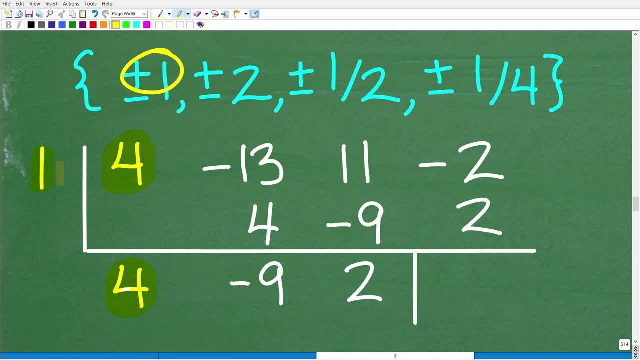 So you're going to drop down this four and then you can take this number one and you're going to take one times four. So what's one times four? That is four. You're going to put your answer in the next column. All right, Now you're going to add down negative 13 plus four is what. 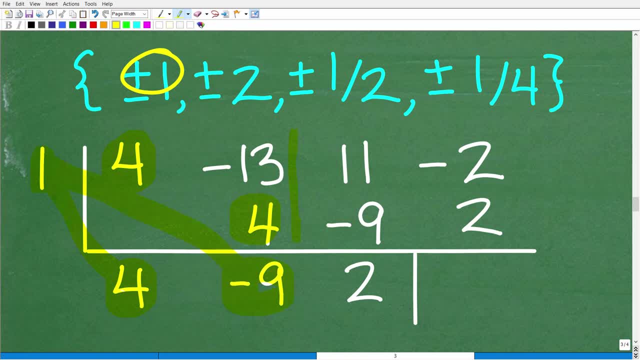 Negative nine. Now you're going to multiply again One times. negative nine is what That's negative nine. You're going to put the answer in the next column. Then you're going to add down 11 plus negative nine. Negative nine is a positive two. 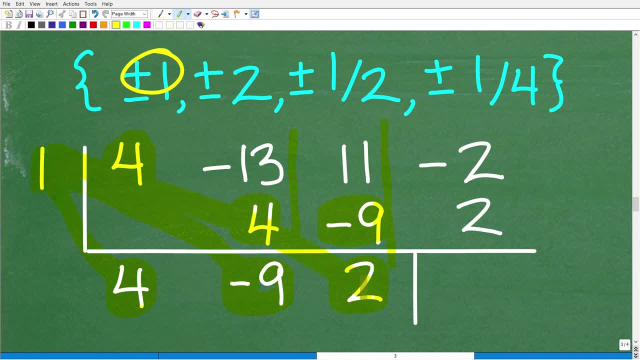 OK, so then we're going to do the same thing again. So one times two is what That's two, Put it in the next column. And negative two plus two is what It is zero. OK, and this right here is what we are hoping to get. 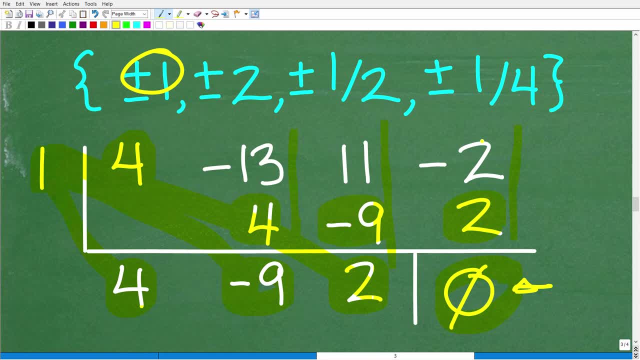 So if you have zero as the remainder, or if you get a zero as your last number, that indicates that this number here is in fact a solution. OK, so this is a much easier way to check solutions And then just plugging in that number. both are equivalent. 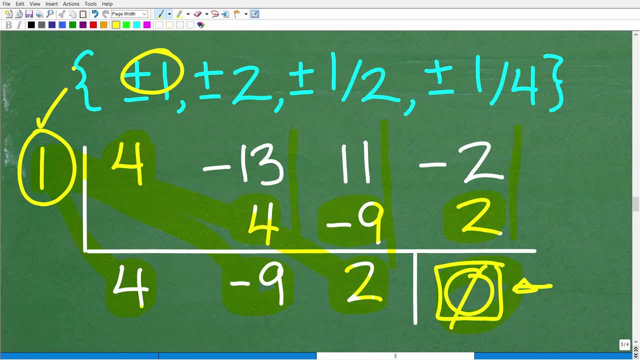 But you've got to understand synthetic division, All right. So hopefully you understand what I did. We'll take a look at another couple problems. But here is something even cooler- I would say cooler, just as cool or interesting- about synthetic division. 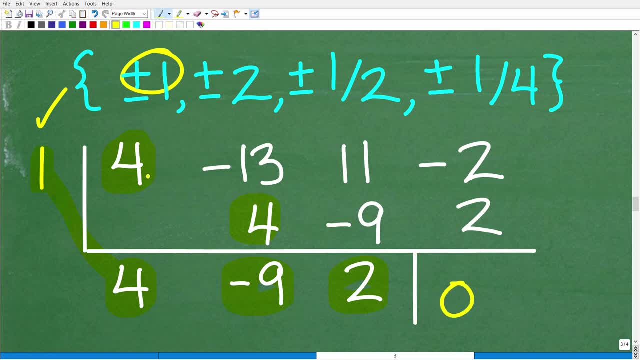 All right, Now here remember four. four was the coefficient in front of our X cubed, And then negative 13 was a coefficient in front of X squared, And this was in front of our X And this was our number. 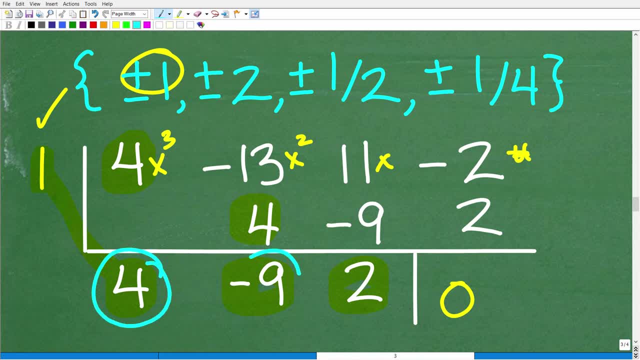 All right, Our answer now? our answer is these here: OK, what happens is you go down a power. So this four: if I want to kind of rebuild this polynomial seven, X cubed, this would become X squared instead of X squared. 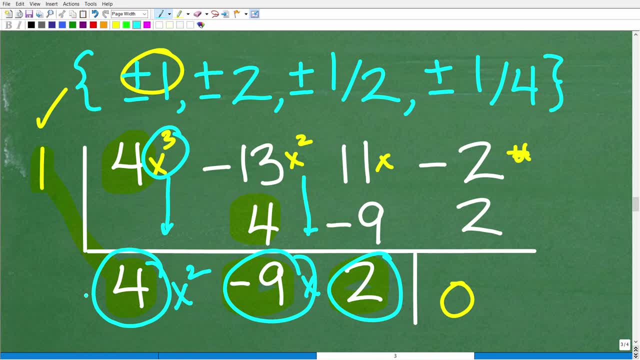 This would become X, And then this X becomes a number. So this right here for X, squared minus nine, X plus two. I know it's kind of hard to see that, because I kind of wrote that We can figure Out the rest of the solutions because this is a quadratic equation. 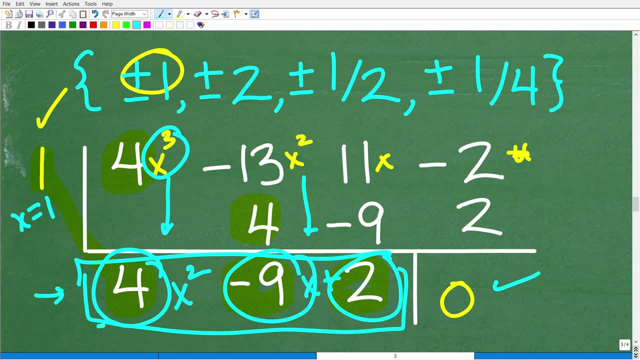 So we know that X is equal to one is a solution, because we've got a zero here. Now here I can go through and figure out the rest of the solutions by solving this quadratic equation. Or I can continue on using synthetic division, using these coefficients, right here. 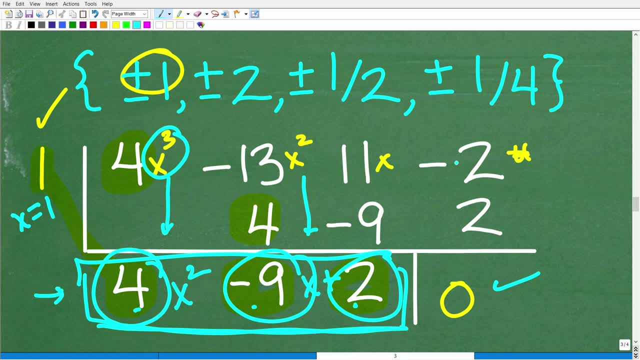 OK, so you've got some options, or you can use these coefficients. Now, technically, what you're supposed to do is take this one and then check for double roots, something like: hey, Mr YouTube man, don't forget to say. 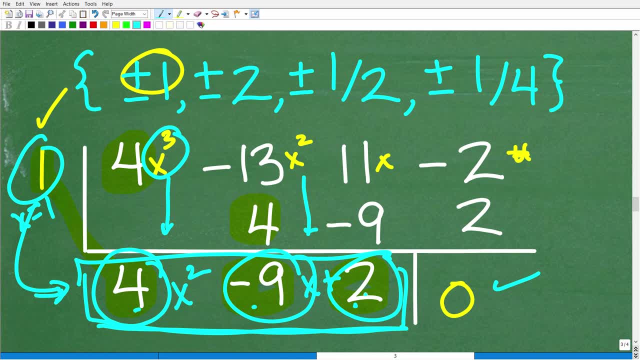 About double roots. Yes, Again, you would take this one and you can check again, All right, So this is a big, big topic. Again, I'm just kind of, you know, doing an overview of this. I know there's a lot of information. like boy, my brain hurts. 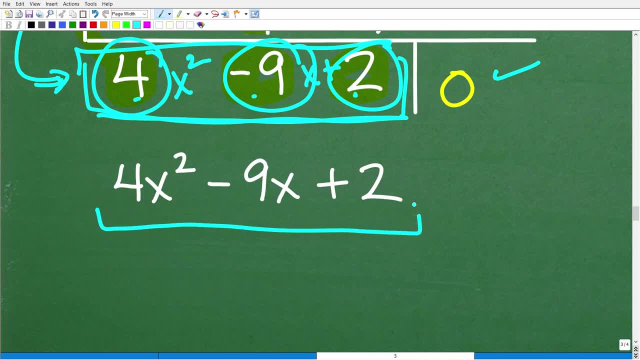 So let's kind of continue on. So here is our other remaining polynomial. OK, so in fact, because X equals to one is a solution, we can even write that as a linear factor: X minus one, this is equal to zero, And this times this, because X is equal to one, is an answer. 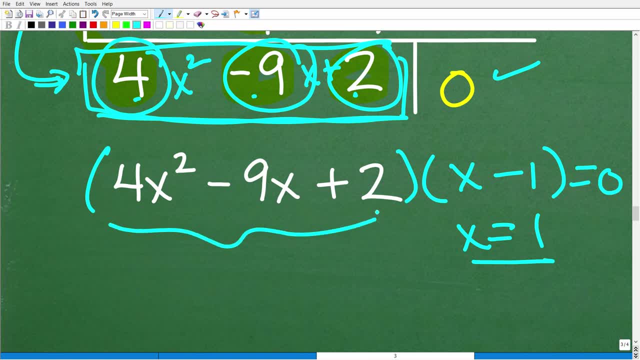 So now I could just figure this out using the quadratic formula or factoring or whatever the case is, And I would have my other X answers and my other solutions. OK, but let's go to continue on and practice synthetic division. So, as I indicated, you can continue. 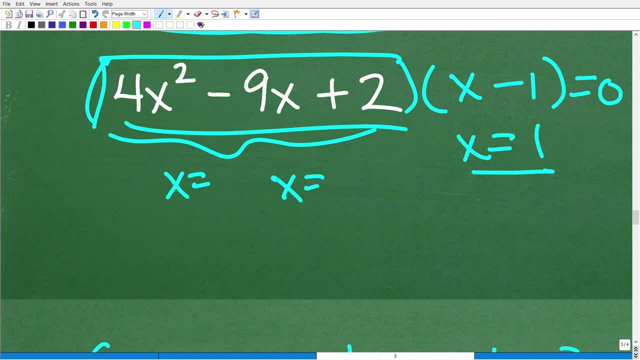 to check for rational roots by just using these numbers. We don't have to use all the numbers in the original polynomial, So we can check with four negative nine and two. Again, these aren't standard form, So Let's go to practice. 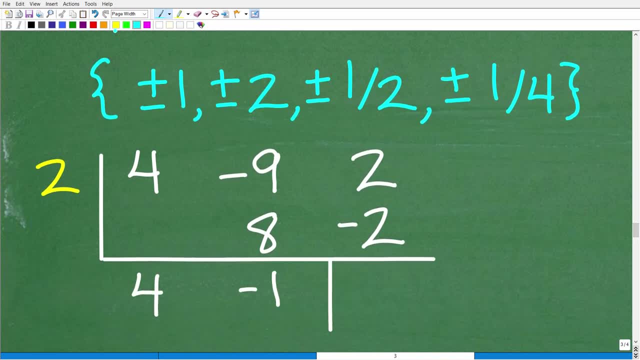 So we got four negative nine and two, And so what's going to happen is this: We checked positive one and then you're going to check negative one. You would see that that's not a solution. And now we come across two positive two. 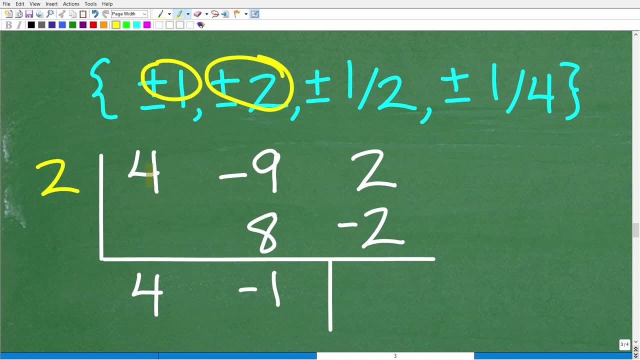 So what's going to happen when we come across positive two? Well, we're going to do this again. So four, we're going to drop that four down Two times four is what? eight and down, and we're going to put that answer in this. 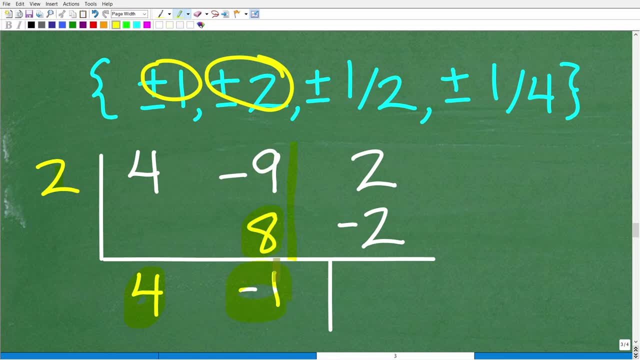 column: negative one plus eight is what? negative nine plus eight, excuse me, is negative one And now we have two times negative one. is what? Put that answer over here? Negative two, two plus negative two is zero. OK, meaning that X is equal to two is a solution. 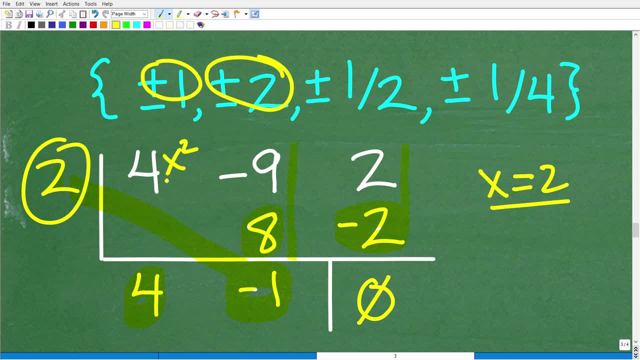 So if this was X squared- remember this is coming from this quadratic trinomial that we had for X squared minus nine, X plus two. Well, we're just going to go down one. So this is four X, This is X. 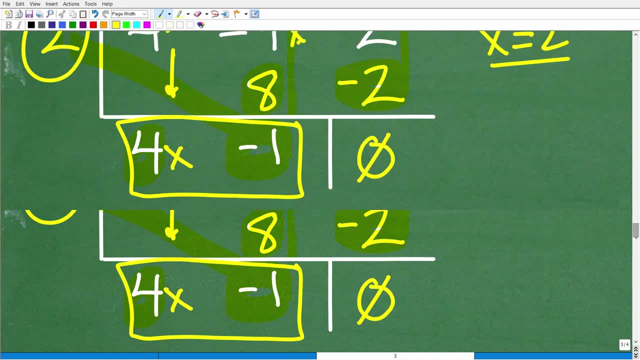 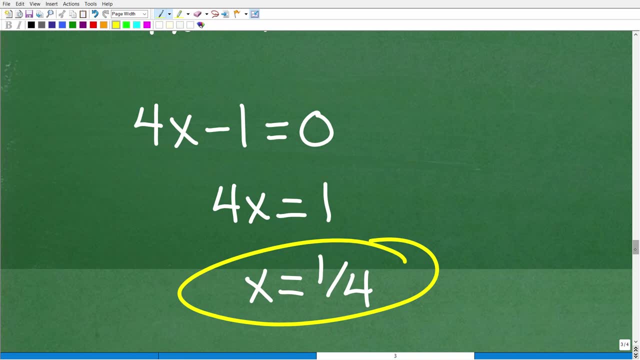 This is a number. So now we could just solve the equation of X minus one equal to zero, And you can see, when I do all this math I get X is equal to positive one fourth. Now, positive X is equal to positive one fourth is a rational number. 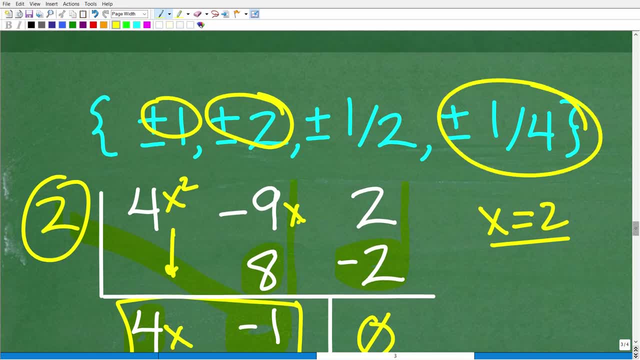 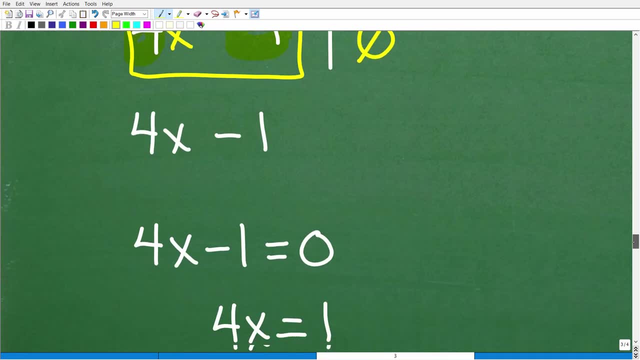 But look, it's also in our list. So all this makes sense, And of course, you can plug in these rational numbers and test them in the original polynomial. There's a lot of different options that you have, OK, so now, what does this all mean? 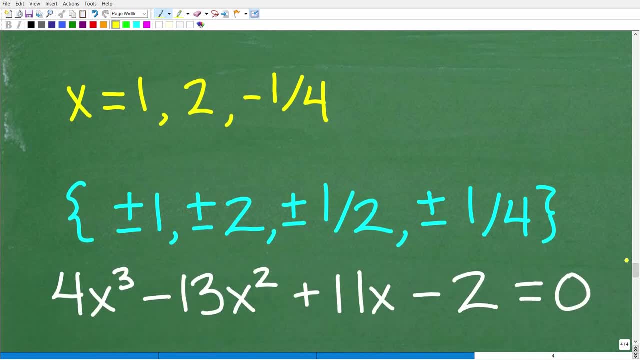 Well, it means that these are the solutions, and we're pretty lucky To have all rational solutions for this particular polynomial equation. Certainly, it's not going to always be the case that you have all rational. you know zeros or roots, So here is the main idea. 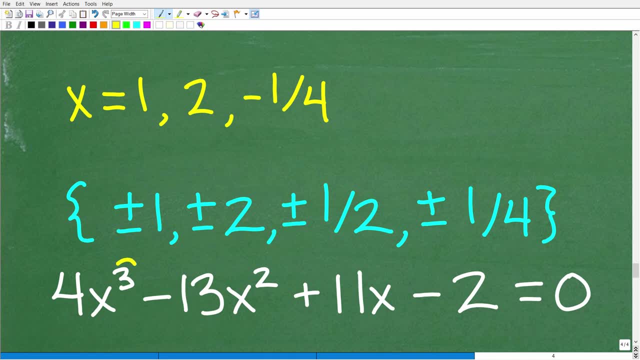 When you're facing a polynomial equation, a third degree or above. OK, you're going to need some other big tools to solve these equations Right. So what are they? Well, one: if you have the graph, that is awesome. 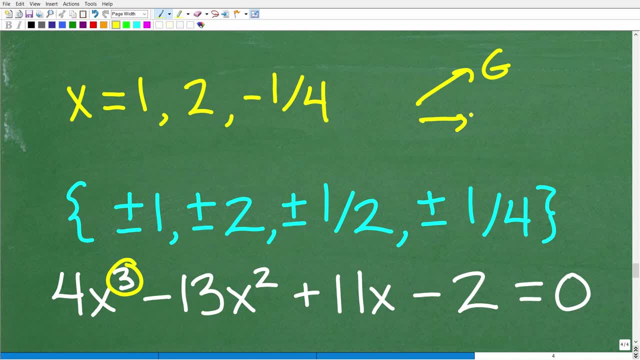 That will give you some clues And if you want to know why you got to check out my full instruction. But graphically we can kind of locate where the roots are going to be, And having a graph is tremendously powerful and useful. 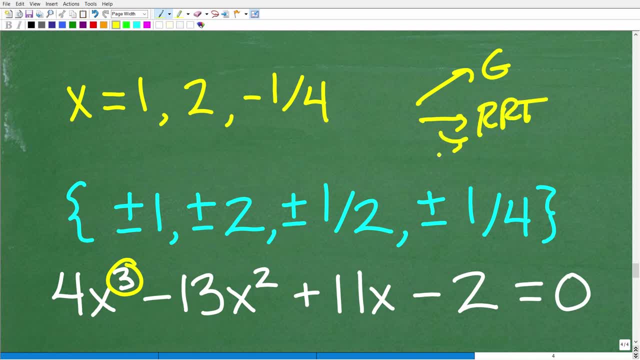 But beyond that we have the rational root there. But then you have other things called like Descartes, rule of signs, et cetera, et cetera. So you have a lot of different things that can help you out. But solving these equations are not so easy. 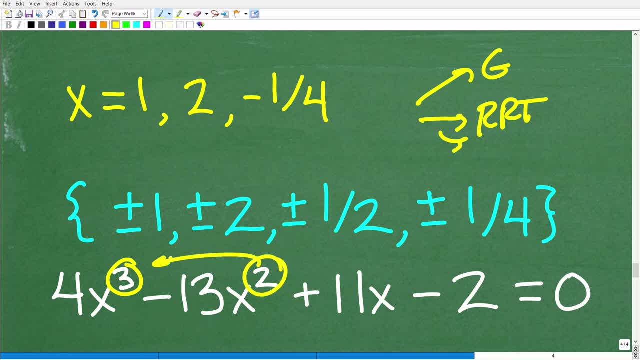 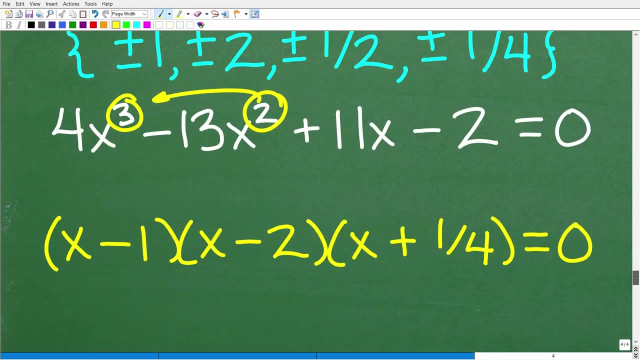 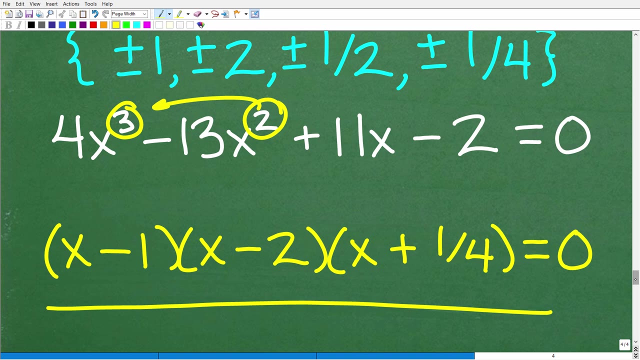 So it's a big jump up from just a quadratic equations to a third degree. it's a whole nother realm. Also, you can write this entire polynomial. You can factor it into what we call linear factors. So our answers were one two and negative one fourth. 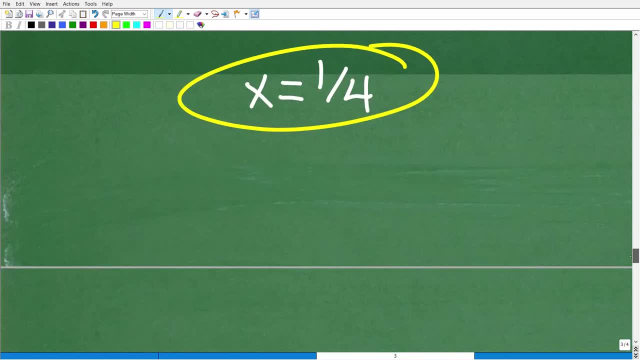 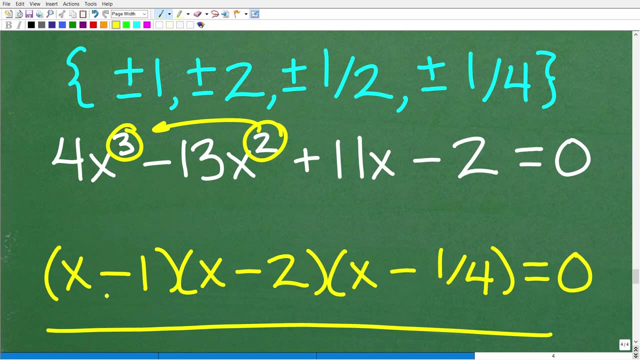 Right, So let me just make sure that was a positive one. fourth Matter of fact, I have to fix this right here, So this is going to be negative. I kind of notice that. All right, So we have X minus one times X minus two times X minus one. fourth is equal to zero. 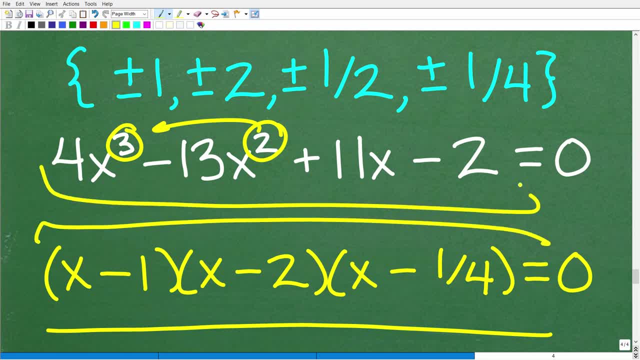 So these would be the factors Of this. So if you wanted to factor this, you can try to factor it by finding these rational roots. OK, so a big topic, And just imagine this is just an overview of this one problem in terms of level. 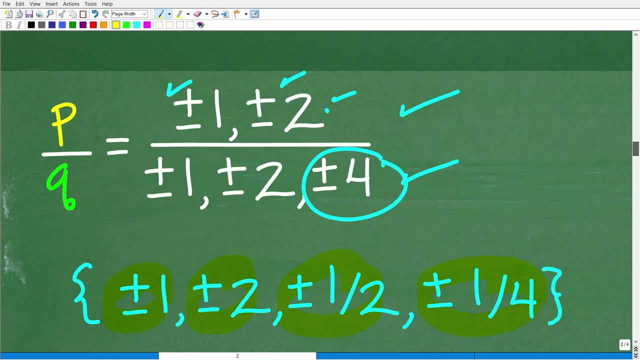 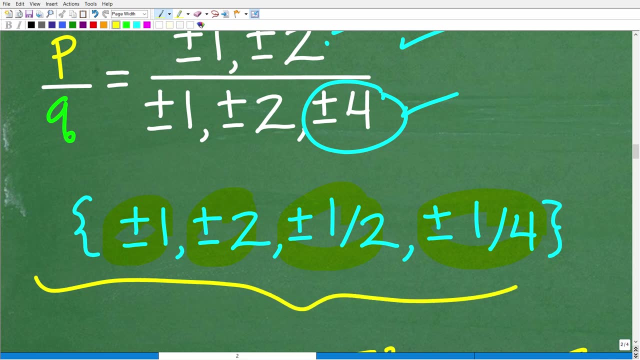 of difficulty. this is not all that difficult of a problem because these P's and Q's, these lists right here, this list right here, there are problems Where, what do we have here? One, two, three, four, You know different positive and negative, positive and negative number options. 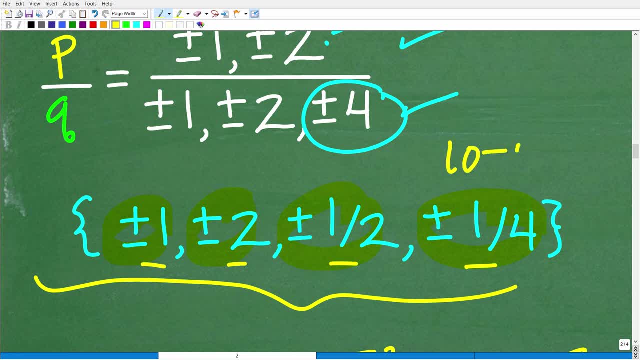 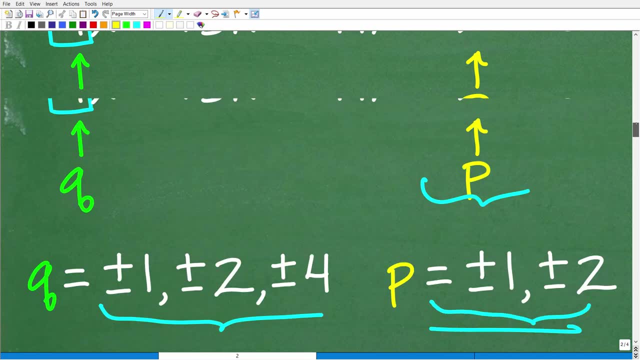 You can easily run into problems. We have like ten, fifteen different possible rational routes. That's where you definitely need to kind of use those other tools that we talked about, like graphing, et cetera, et cetera. So a big topic, lots to cover. 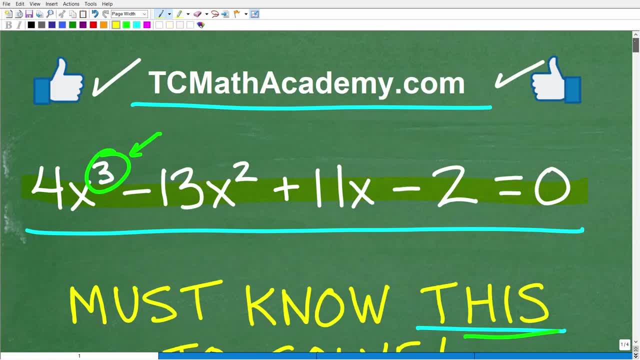 And if you don't understand everything that is understandable. So just you know, use this feedback or use this video as feedback, Right, But hopefully this you know kind of helps clear up some of these things. that again, if you're at this level of math that you 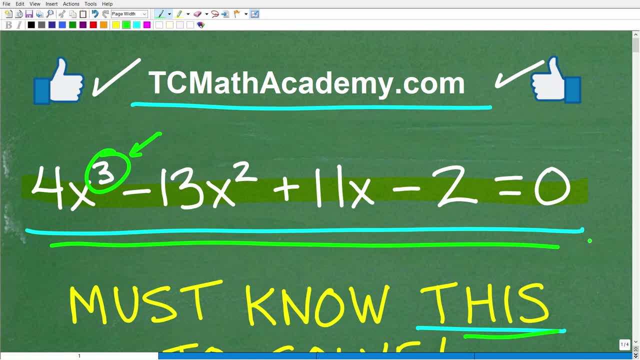 need to know, so don't feel bad if you're like boy, this is, like you know, a lot of work. Yes, indeed it is, But you can definitely do this and hopefully this little video helps you out. And if that's the case, don't forget to like and subscribe. 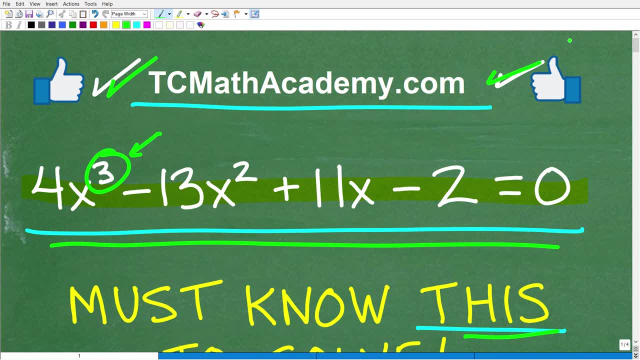 And, with that being said, I definitely wish you all the best in your mathematics adventures. Thank you for your time and have a great day. 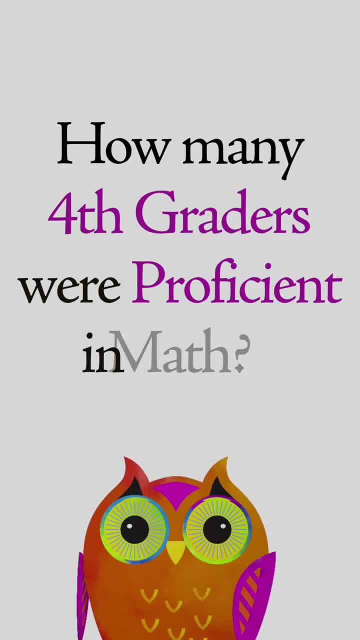 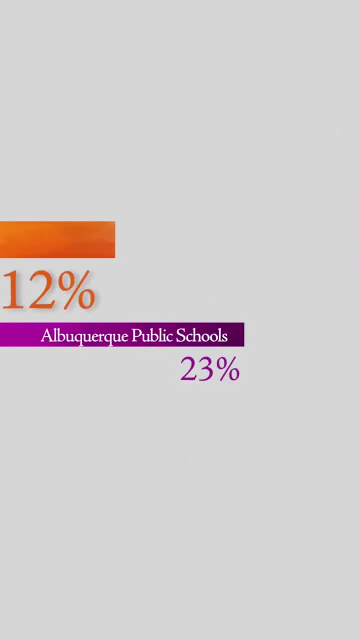 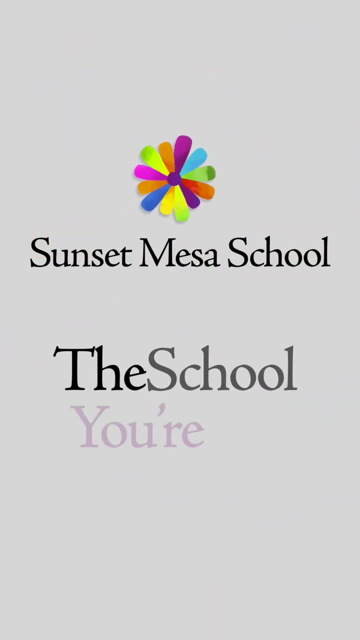 Last year how many Albuquerque fourth graders were proficient in math? Albuquerque public schools- 23 percent of students, but Sunset Mesa school- 100 percent were proficient. Sunset Mesa might be the school you're looking for. We're an academic pre-k and elementary school. 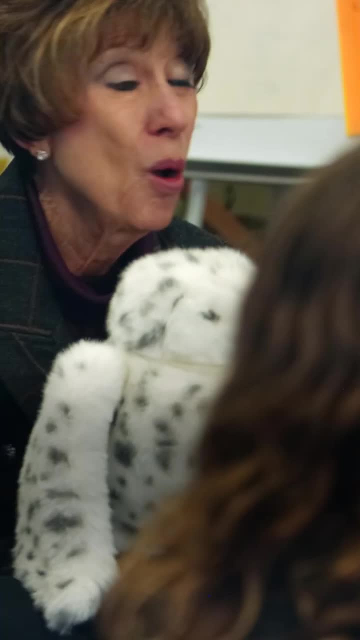 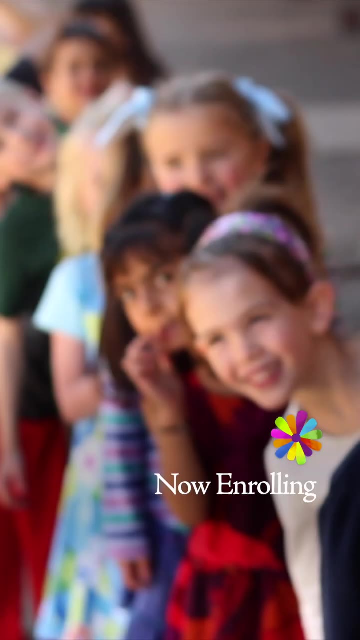 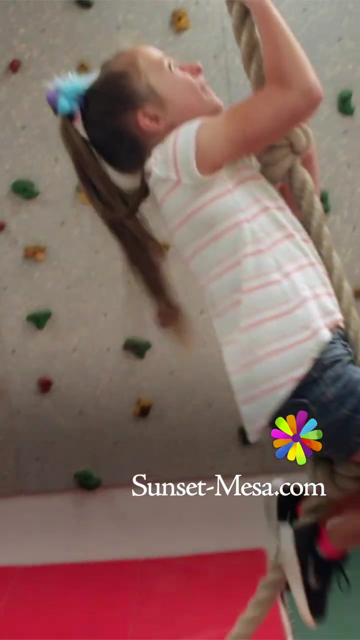 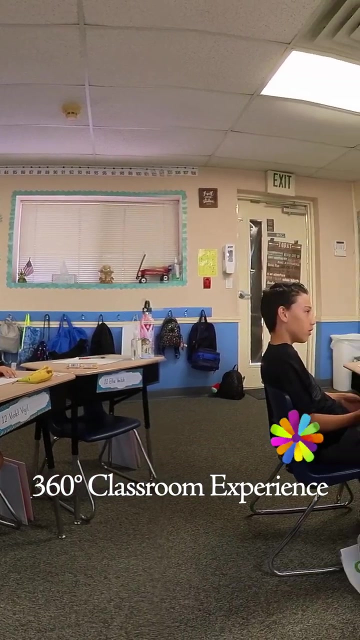